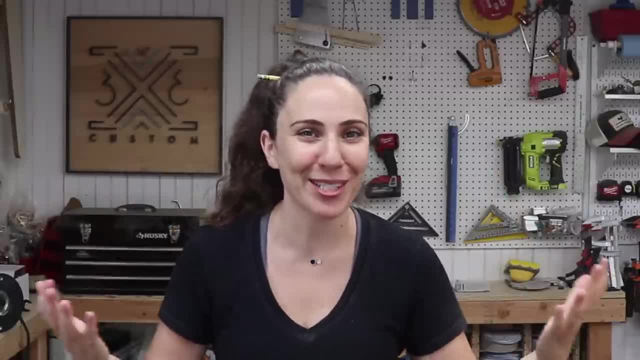 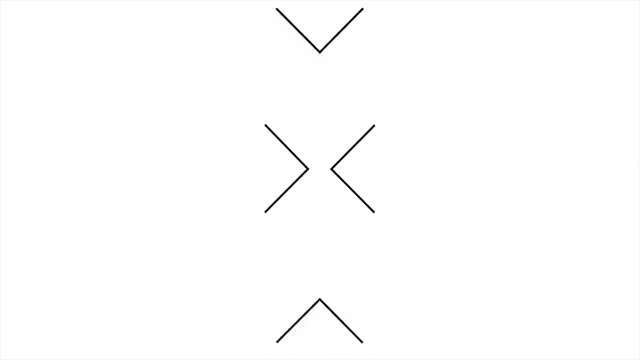 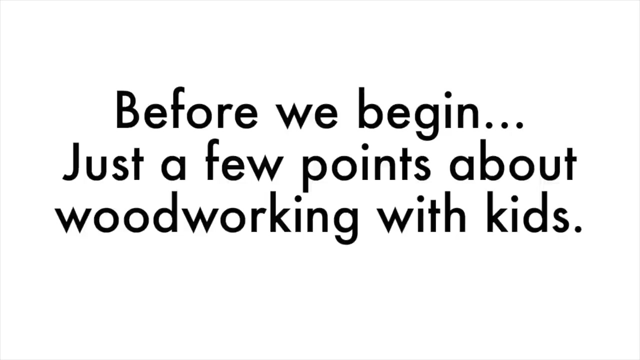 Since a lot of us are stuck at home with our kids this summer trying to come up with stuff to do with them, I figured I'd make a video on some quick and simple woodworking projects that you can build with your kids. Number one, and most important, is safety. I cannot stress this enough. 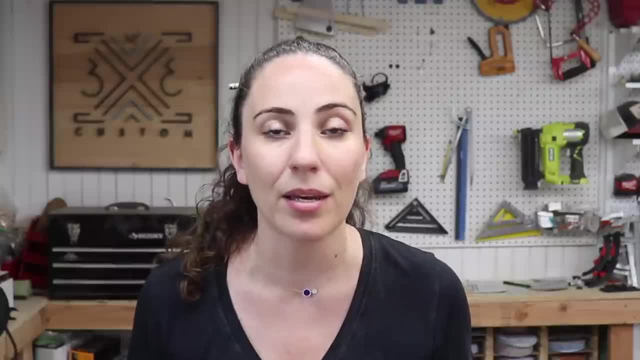 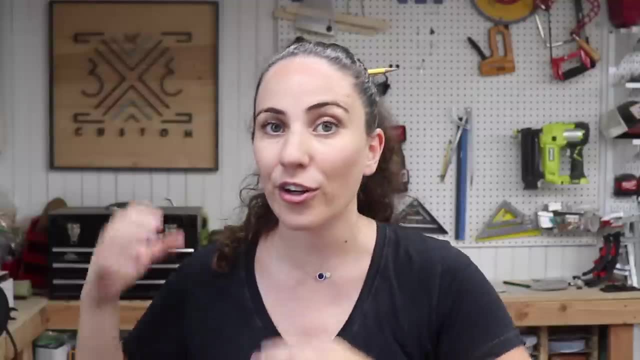 Obviously, the entire time your kids should be wearing the proper PPE, but also you have to determine which tools you're going to let them use, And it's going to vary from kid to kid. There are some 16-year-olds who cannot focus at all and cannot listen to any instructions. 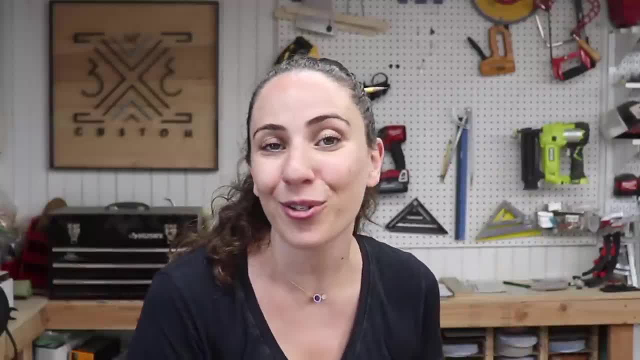 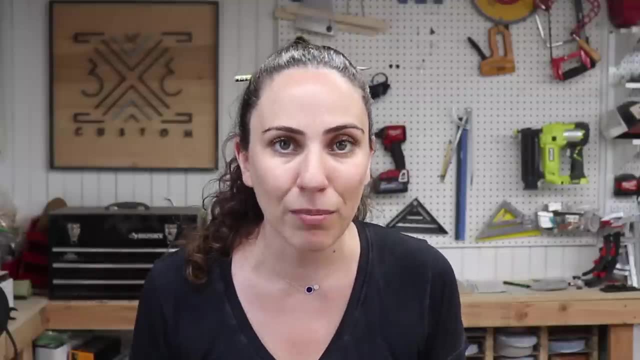 so I wouldn't let them near any tools. Yet there are some eight-year-olds who have a laser-like focus and listen to everything that you say. So you really just have to evaluate your own situation, be smart and make the right decisions for you and your family. I personally do not let 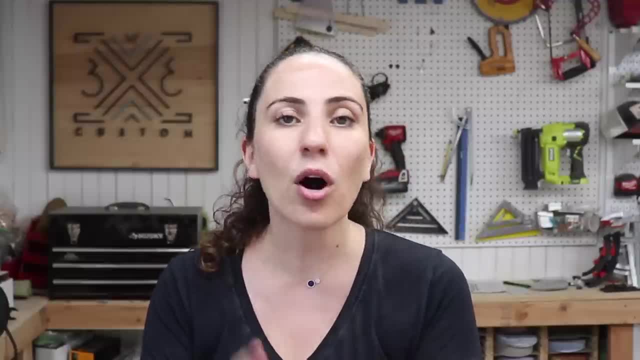 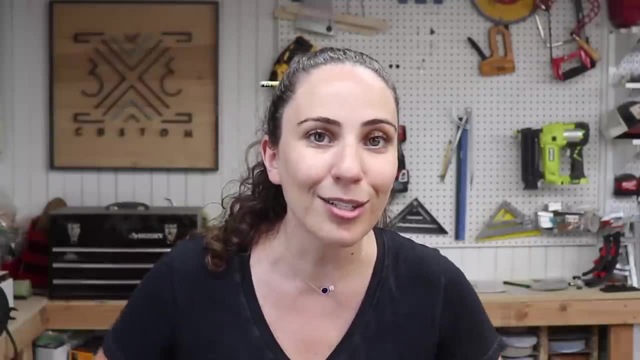 my kids near my table saw my miter, saw my circular saw or my router. I'm not going to be using those tools in this video as the prep work that's going on. I'm also going to be showing it because it's a quicker way and you will be able to get the same. 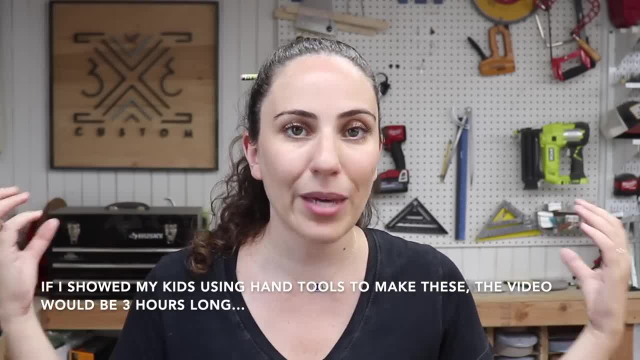 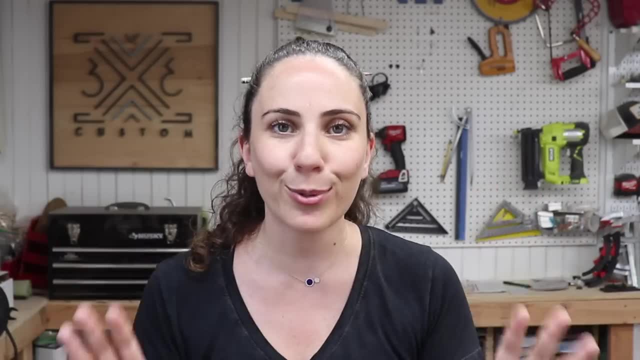 results using other tools around your shop. So I'm not saying that your kids should be using the tools that I'm using in this video. Evaluate everything for yourself and just be smart and be safe. Number two: let go of being a perfectionist. These projects will never be perfect. 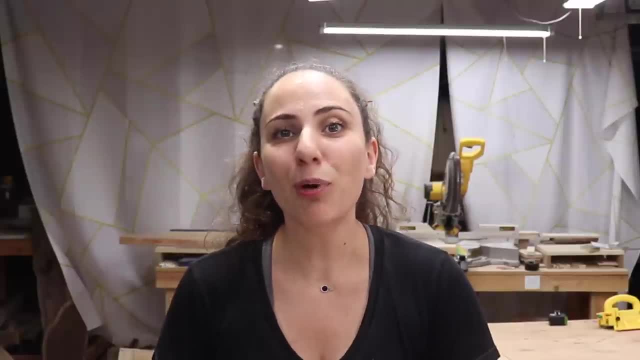 and I'm not saying that you should be perfect, but I'm saying that you should be perfect. Number three: be smart and be safe. Number four: be smart and be safe. Number five: be smart and be safe. Number six: be smart and be safe. 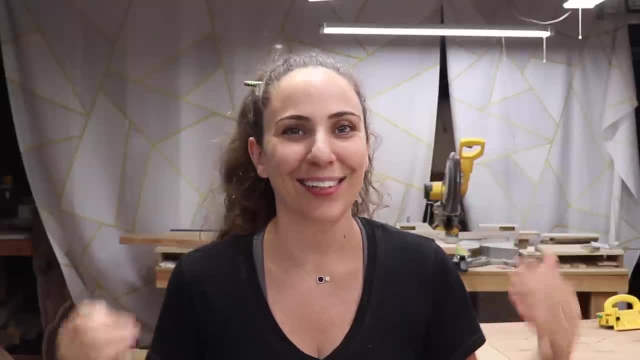 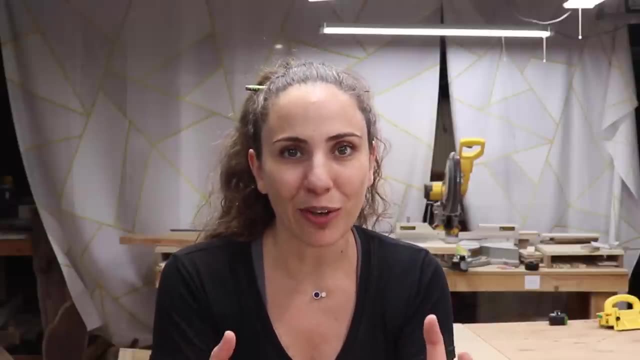 Not be perfect at all And you just have to let it go and let their creativity loose. The kids will not see the flaws in the projects. All they're going to see is something that they actually made with their hands, And when they look at it they're just going to remember the quality time. 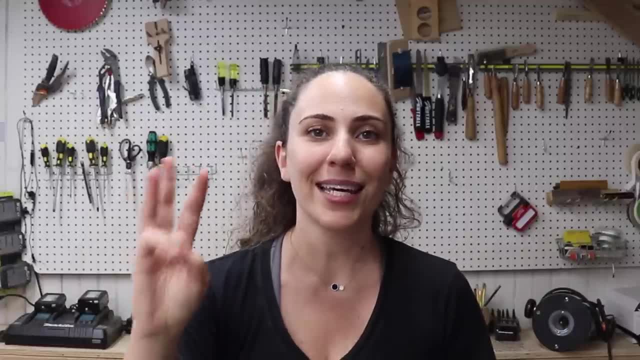 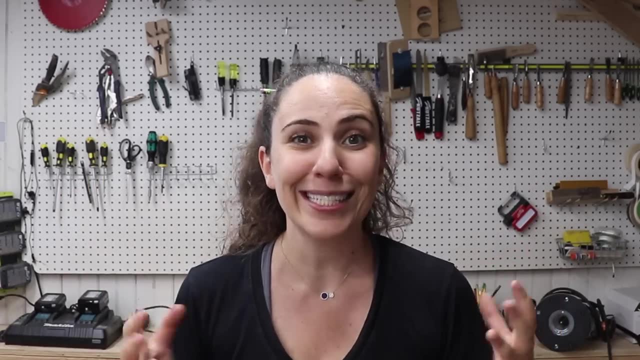 that they spent with you. And the last one, number three: prep is key. So younger kids especially, they just like to see a project come together. So make sure that you make all the necessary dangerous cuts before you get them involved so they don't get bored and just run away. 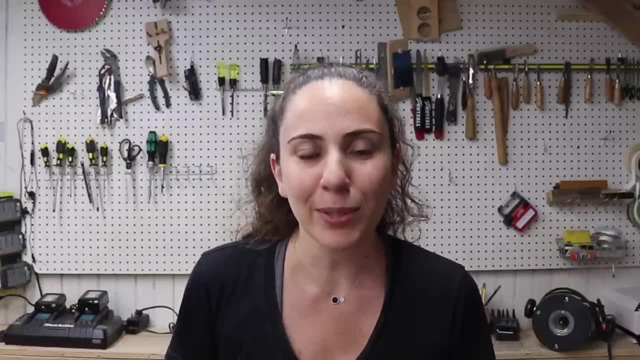 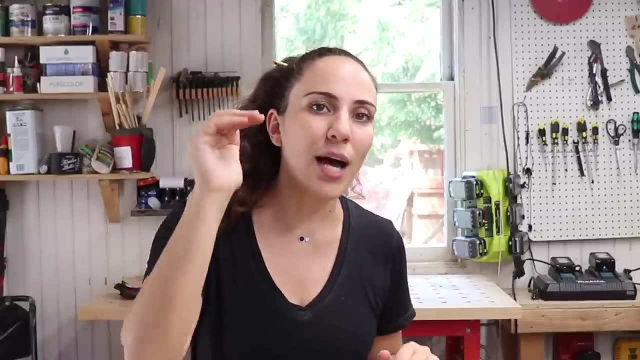 and go do something else. So prepare as much as you possibly can to just keep it lighthearted and fun for them. I'm going to make a few small projects in this video, so I'll make sure to put timestamped links in the description box down below So you could just fast forward to whichever. 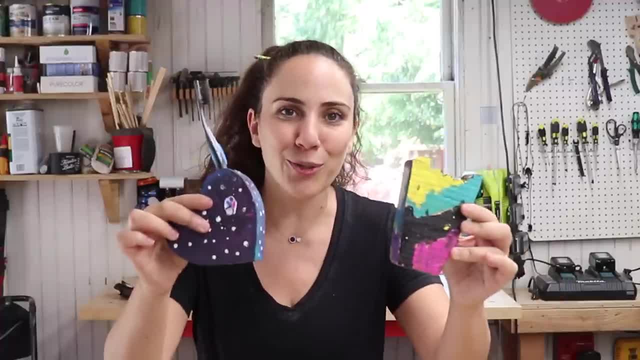 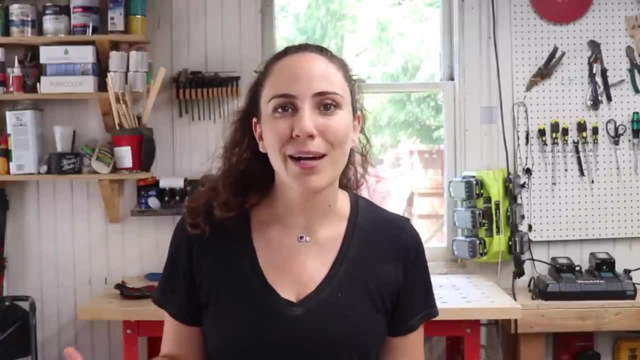 project you want to watch First up. we got these toothbrush holders So you could very easily just print out a shape online and trace that. But I think it's really more customizable for the kids for them to actually draw the shape on a piece of paper. So I think it's really more customizable. 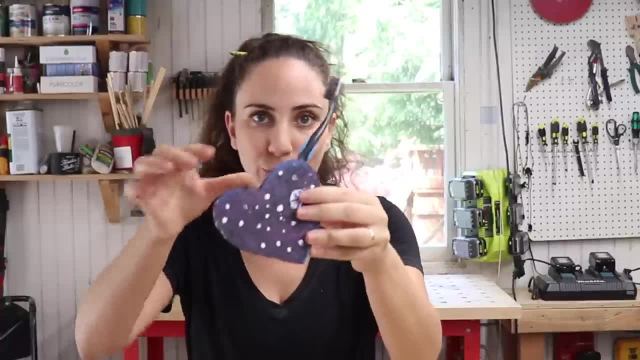 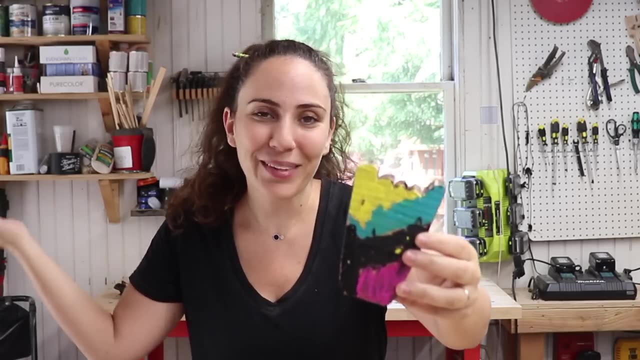 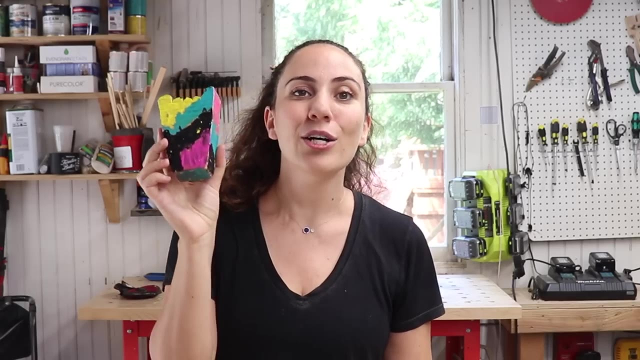 on a piece of wood first. So, as you can see clearly, my daughter drew a heart and my son drew a foot with an extra long pinky toe. Remember, these projects are for them, not us, So whatever makes them happy. I think it's really cool if they draw out the shape that they want and then 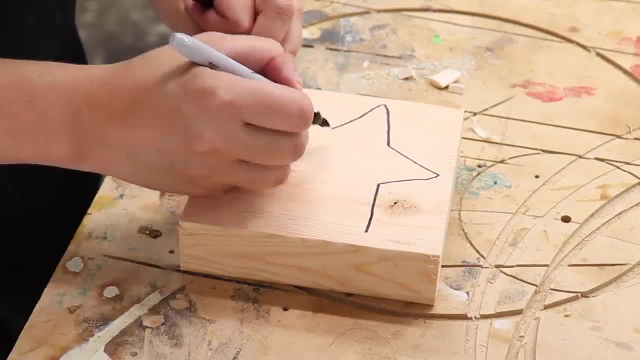 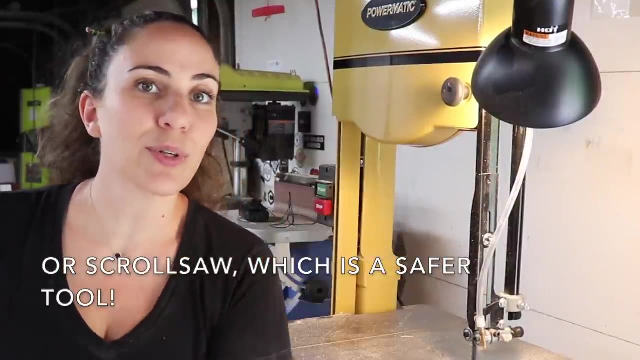 they can see that come alive. Take some scrap tube by material and just have your kid draw any shape they want. Now this could be cut out on a jigsaw or a bandsaw, Depending on how old your kid is. you can actually let them do that part. 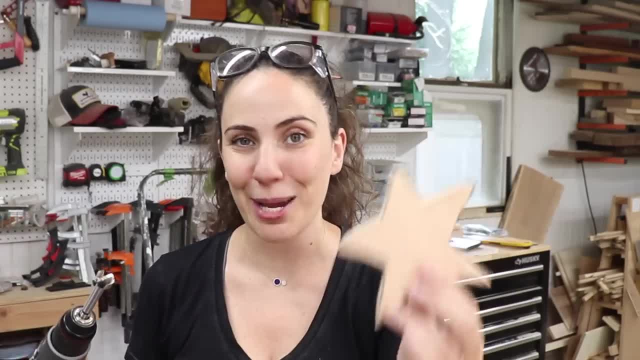 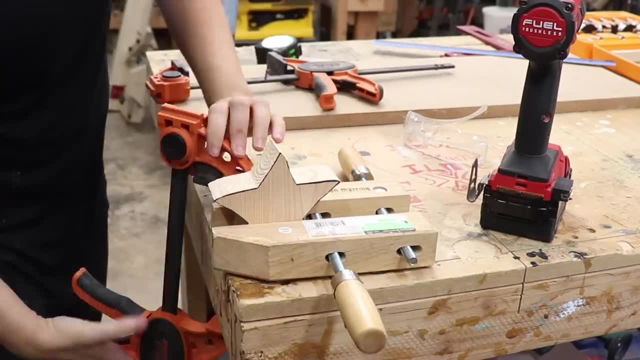 This next part the kids are going to love. They just need to drill a hole through the shape that they created to hold the toothbrush. My kids love using a drill. They love using the drill press. Just got to make sure everything is clamped really well. Now it's really secured in there. 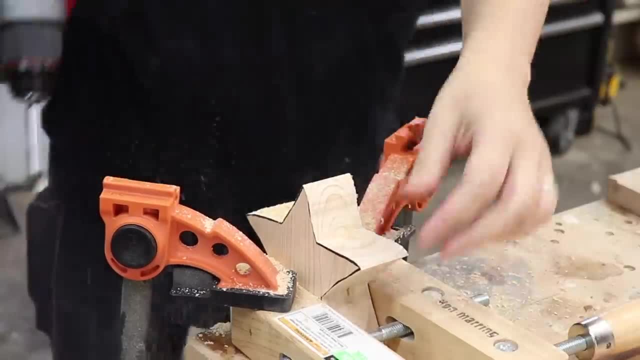 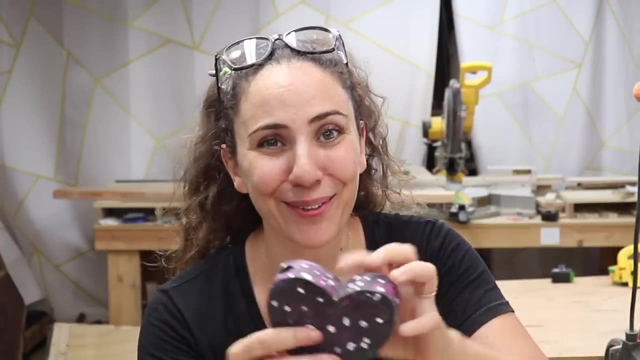 and the kids can safely just drill a hole. I'm going to use sand and paint, which are both activities that kids love to do, and they're done. The next one is a banana holder, So this was actually designed by my daughter, So 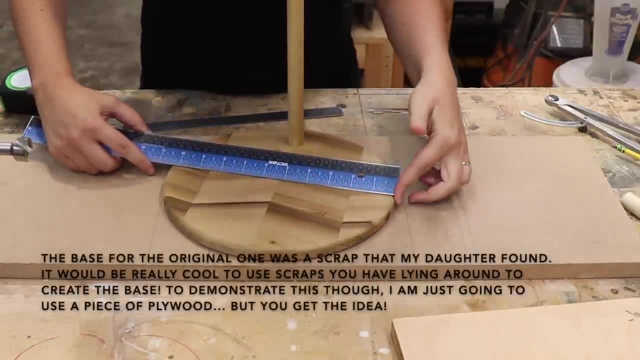 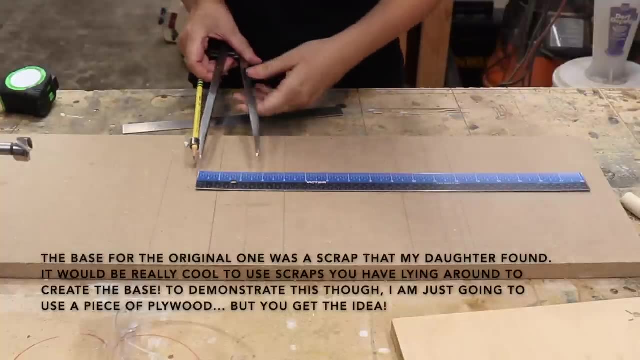 the original one that my daughter designed. the circle's about 10 and a quarter, 10 and a half. I don't think it needs to be that big, So I think nine would be good. So I'll set a compass to four. 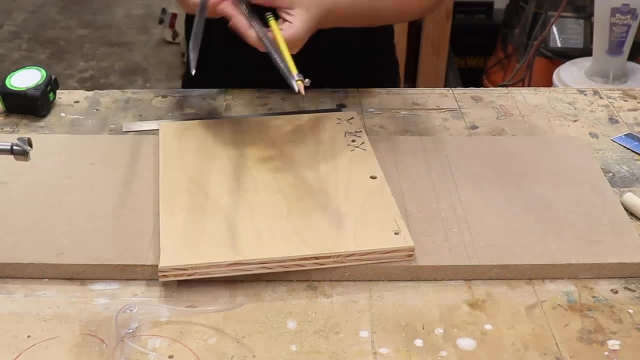 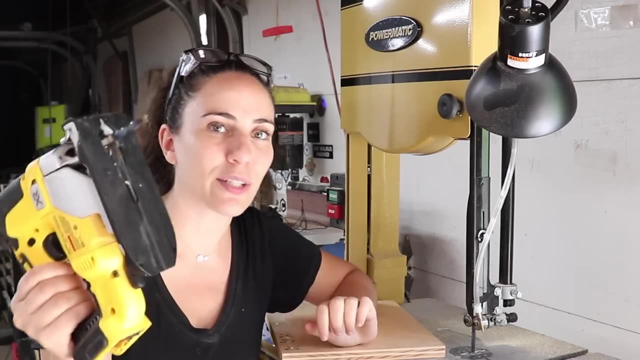 and a half. Take that plywood and just draw out the circle- The original one with my daughter. I actually let her use the jigsaw, So I just stayed right on top of her, always making sure that she knew where her hands were, at all times, Of course. 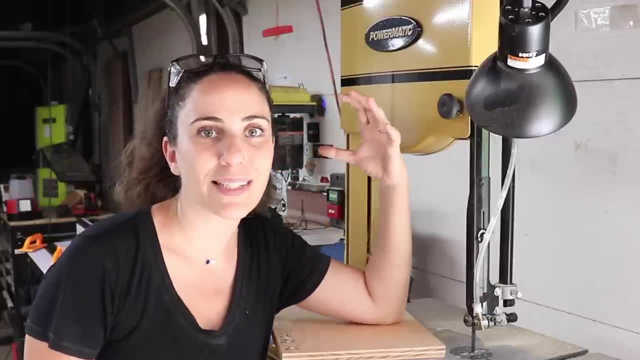 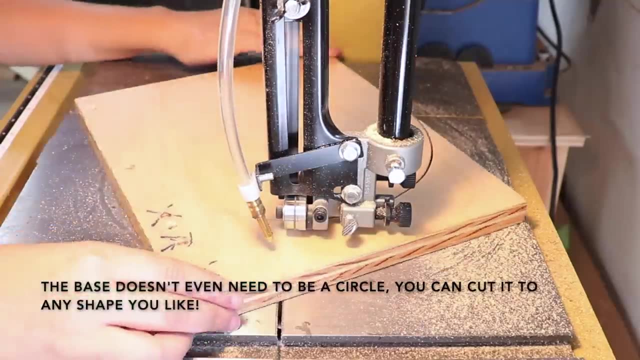 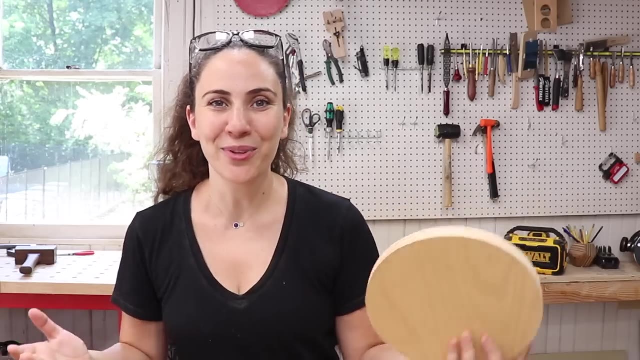 she was wearing the proper PPE and we were able to cut it out really safely. But since this is still a new toy to me, I'm just going to use the bandsaw here Now. the kids just need to sand it smooth, which is an activity that they love to do. The stand. 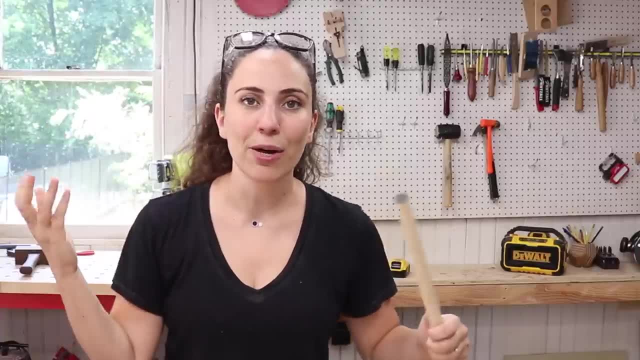 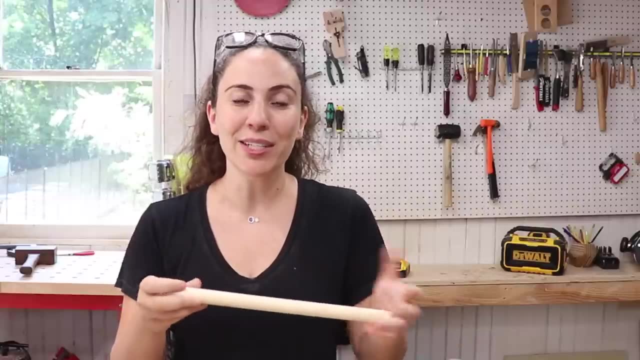 I used a three quarter inch dowel and it was cut to 12 inches long. This is something that's also really fun for the kids to do. They can use a handsaw to cut these dowels and it's really satisfying for them to actually see the cuts happening with a handsaw My kids love using. 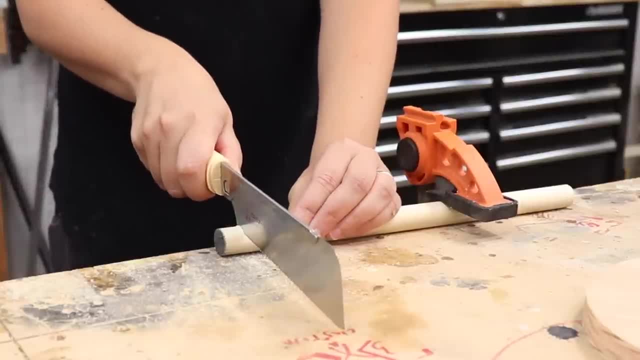 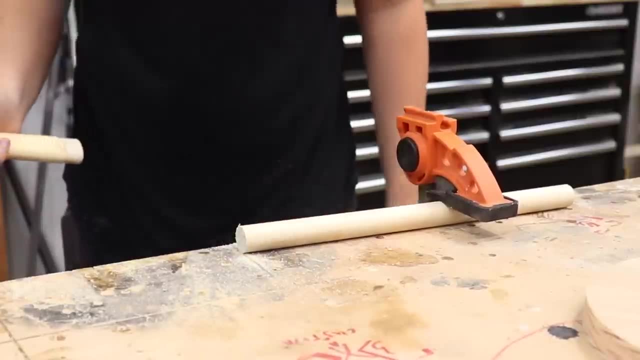 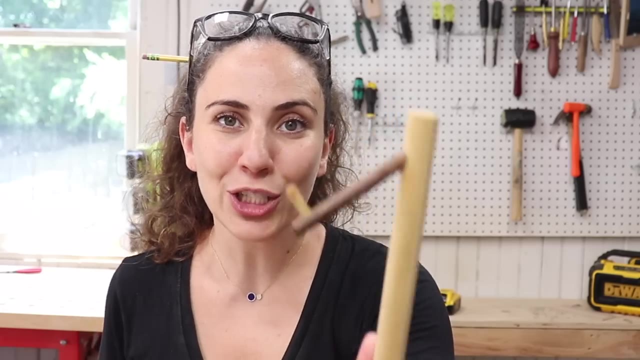 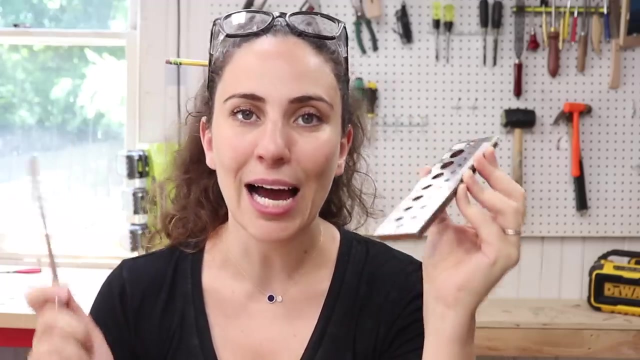 hand tools. This goes really quick: One, two, three, four, five, Five strokes of an adult, probably 10 to 15 with a kid. For the hook part, we actually made our own hardwood dowels using a dowel plate. If you don't know what a dowel plate is, I have a video on how to make. 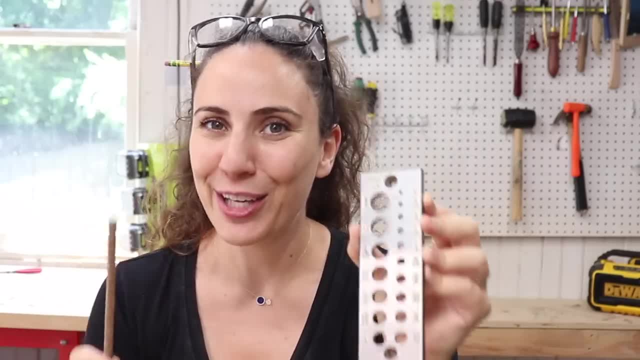 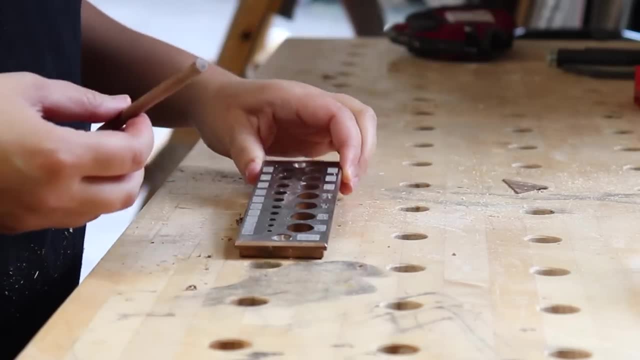 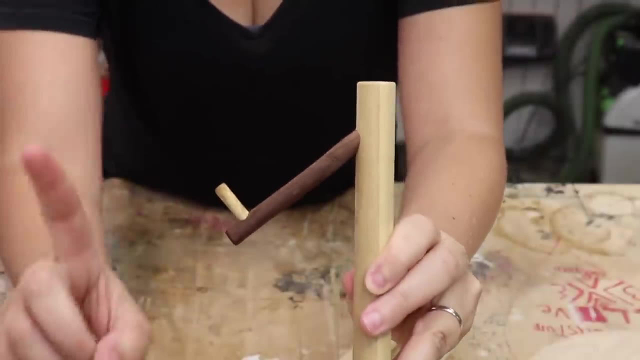 your own dowels, and my kids love using this thing. It's really fun. Basically, it's a metal plate with different size holes that can turn a square piece of wood into a round piece of wood. So, on the original design that my daughter 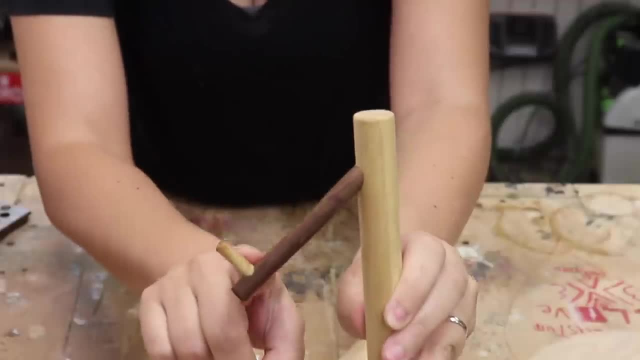 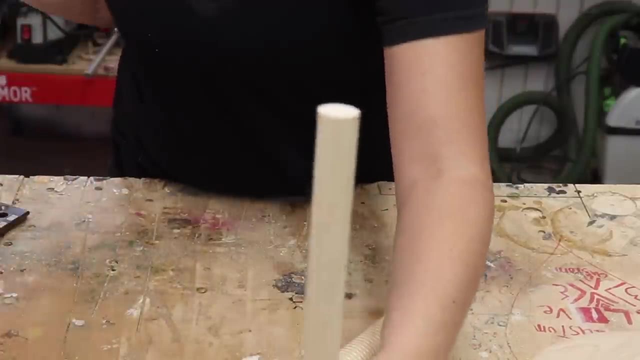 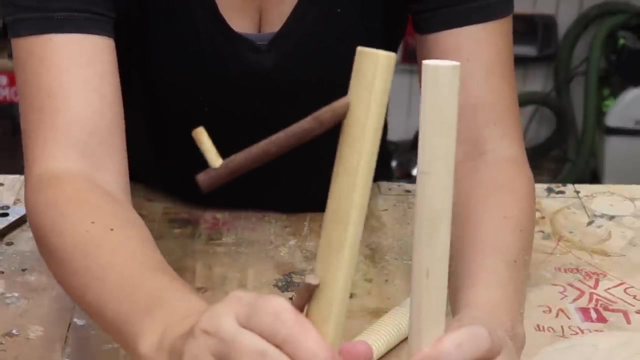 came up with. she made one dowel going down and then another dowel going up, acting as a hook. But I actually think a better idea would be to just install a dowel just facing up instead of facing down. That way you only have one dowel off of your main support here. 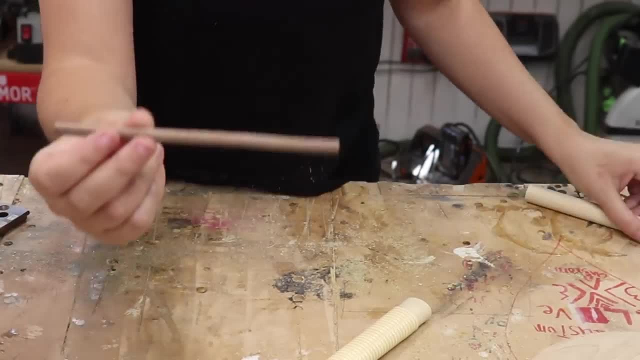 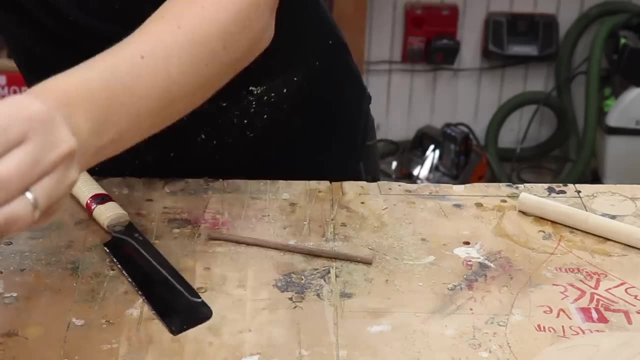 I'm going to just cut this now to length Once again. this is super easy for kids to cut with a handsaw. I don't know how long I'm gonna make this. uh, let's see. four inches seems about right. yeah, four inches sounds right. 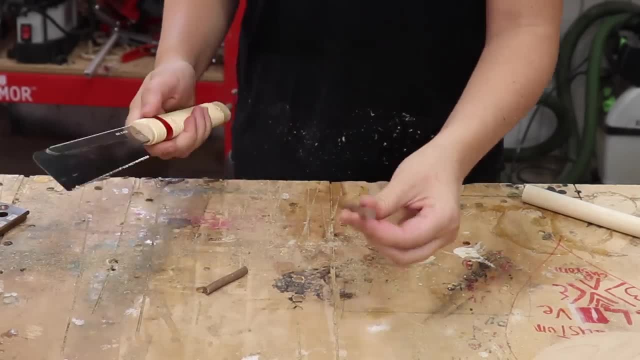 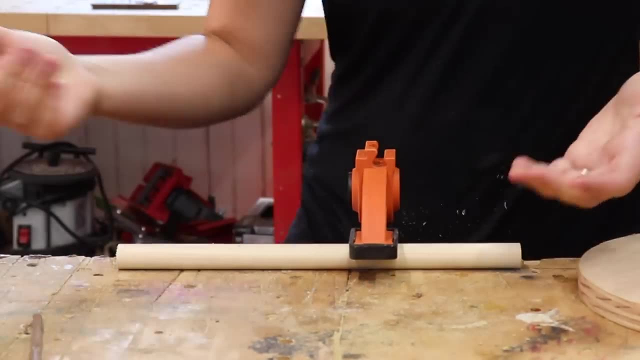 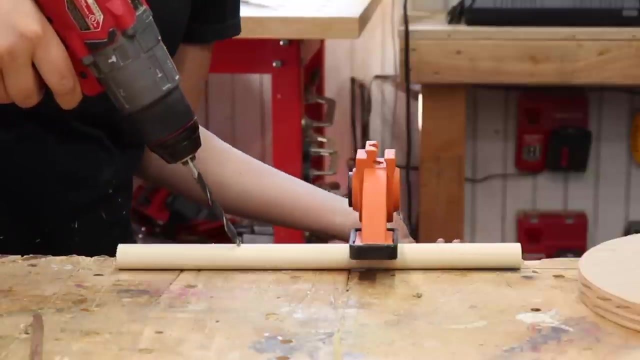 ready one, just one. come on hand saws. yeah, and this is parts that I let my daughter do when, when we, when we made this, just drill into the dowel at an angle that seems like it's gonna work. you don't want to go all the way through. 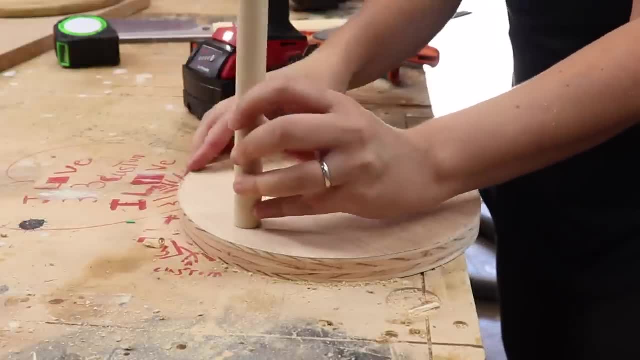 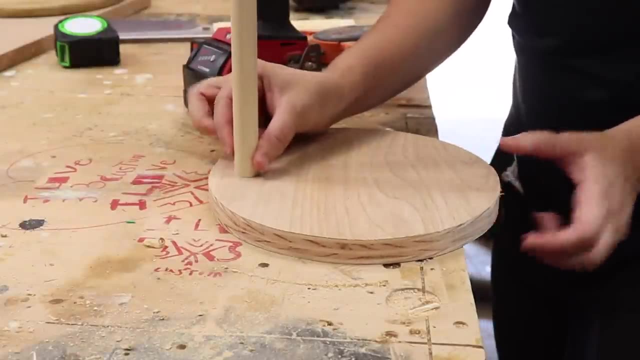 perfect, and now you just want to drill a hole for where to put the standing dowel. you don't want it to be in the center, because that it's going to tip over. you want it to be towards the edge. once again. this location does not need to be perfect at all, just don't want to drill all. 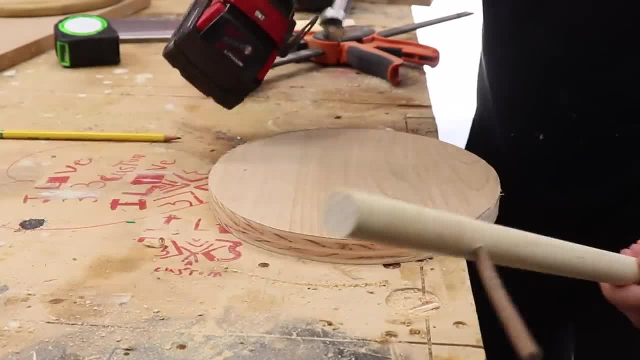 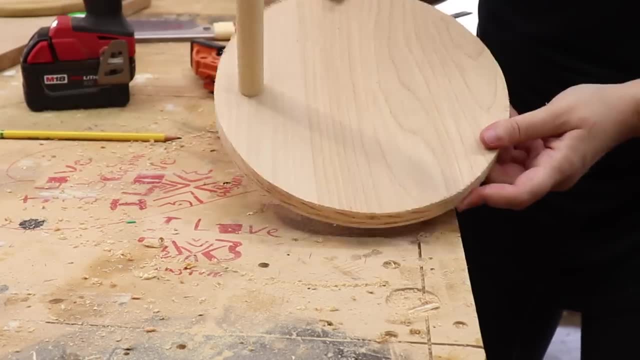 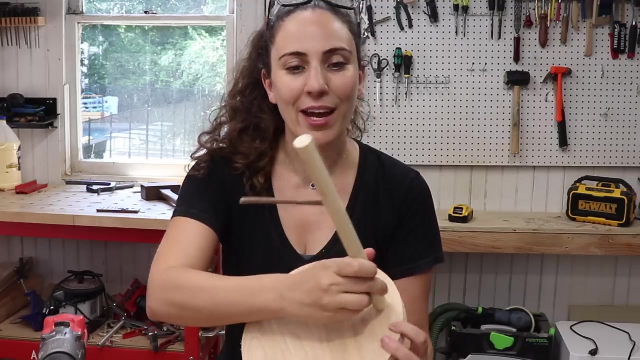 the way through. it's a three-quarter dowel, so I'm using a three-quarter inch forstner bit. that's my new one for this one awesome. next. another favorite step for the kids is to add some glue. so just put some glue in the hole over there. put some glue in this hole over here. 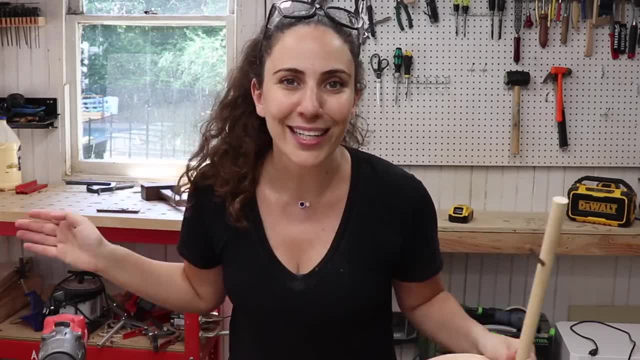 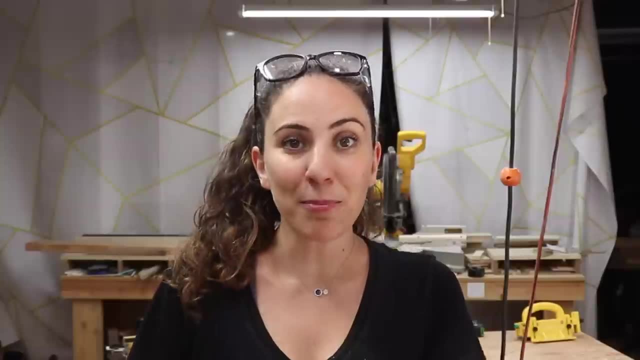 sand it, put some paint on it, put some stain on it, just put some regular oil on it. finish it any way. your kid wants to finish it and I think these look really cool on the countertop and they're really simple to make. next up some piggy banks. so this is actually a project that 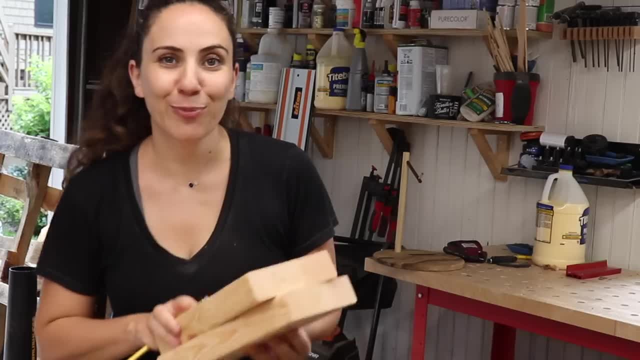 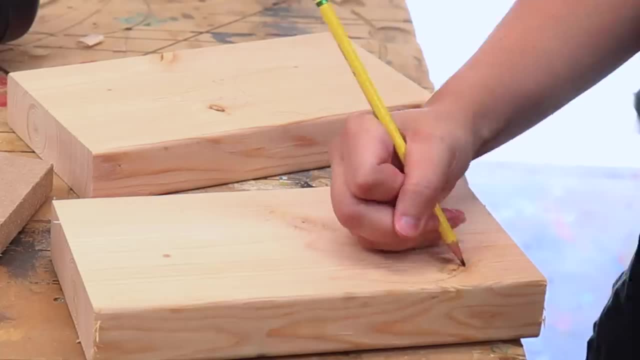 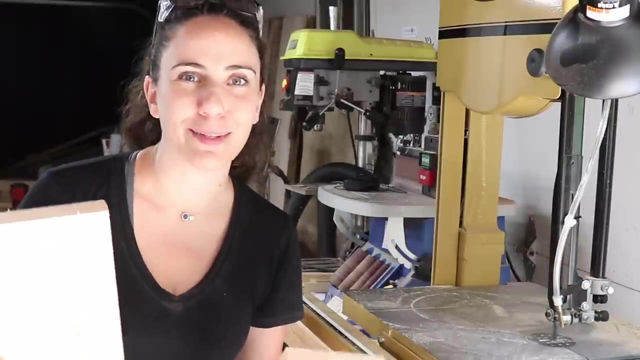 kids before, but that my daughter has been asking for. so i just went inside and my daughter drew a unicorn on this one and i'm going to draw a rocket ship on this one for my son. did i mention that these were two by sixes? i'm not sure if i mentioned that, but 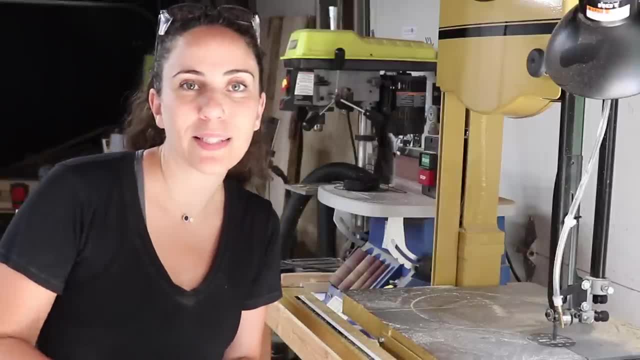 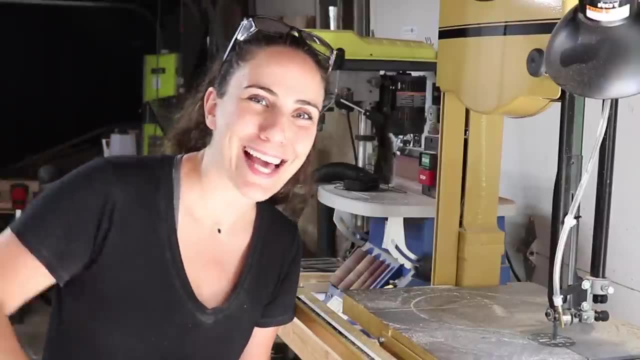 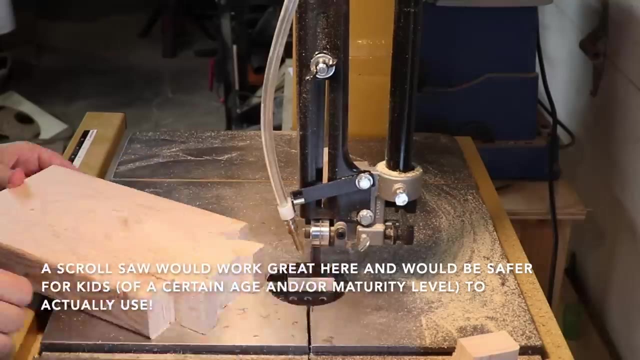 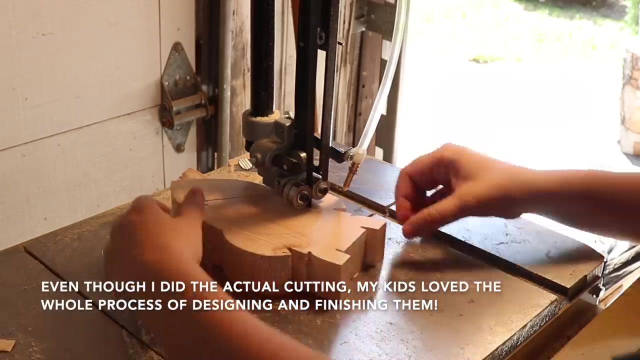 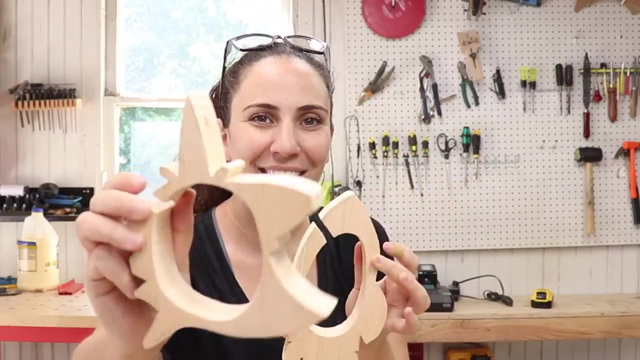 really just use anything you want. you can actually glue up some pieces to make it thicker, but two by sixes, i think should be fine. now, you guessed it. i'm going to cut these out on my new favorite toy, and i cut out that unicorn, just like i cut out the rocket ship. got a little bit thin over here. 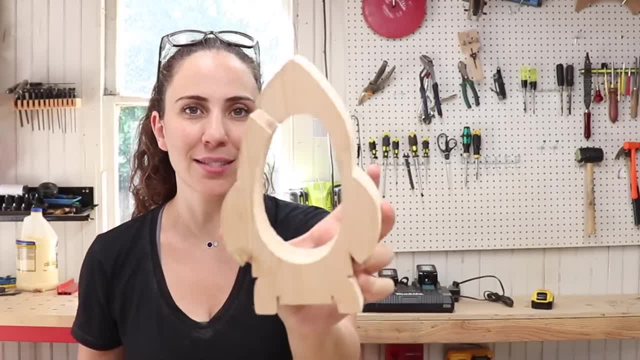 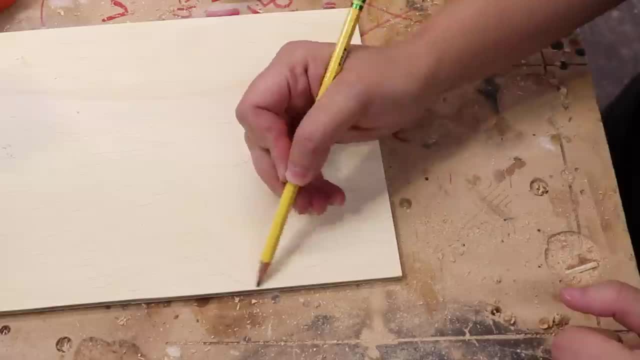 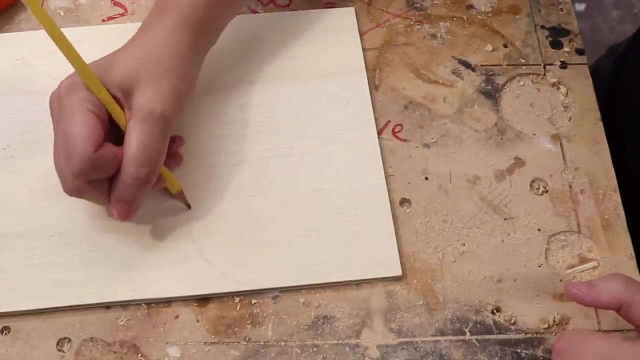 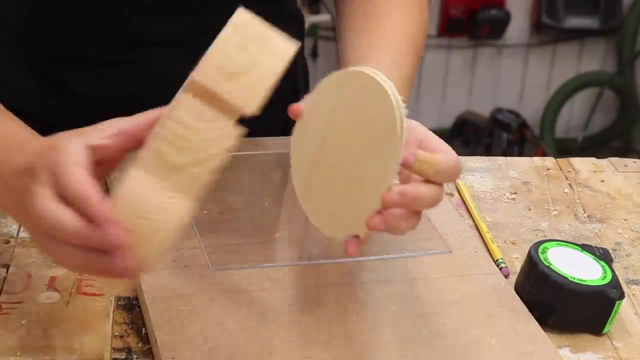 a little bit thinner than i would like, but it's all going to be reinforced in a second. this is would be a better thickness. now i'll just want to draw another circle around that probably like a quarter inch larger. i'm just gonna roughly mark it out. i did the same thing to the rocket ship. 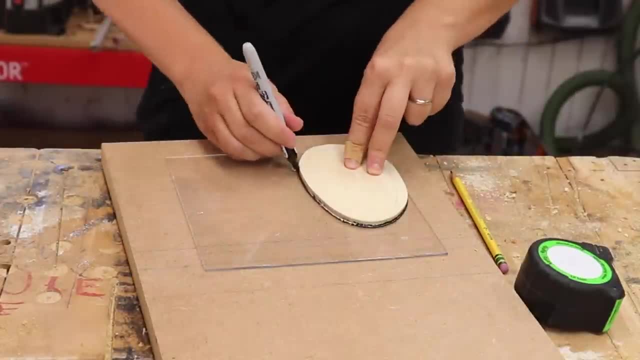 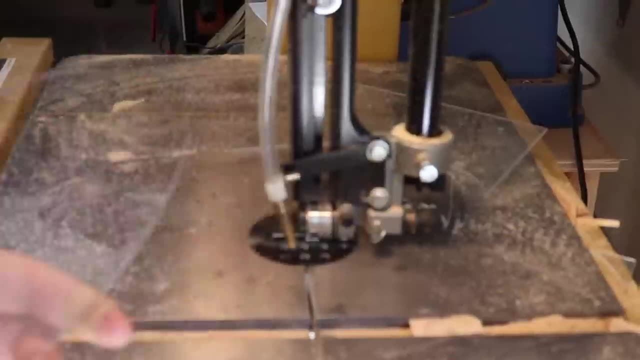 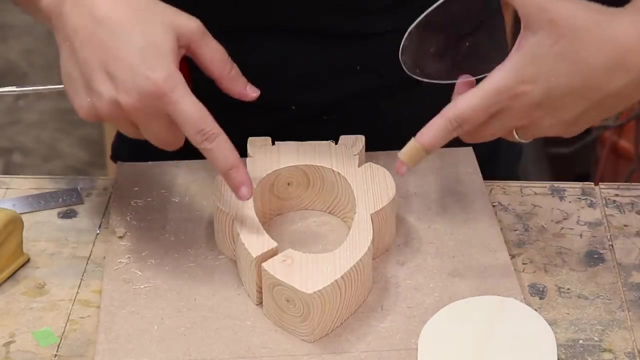 and now that i have the perfect shape that i need, i can just trace that onto the acrylic ground and turn it over. as you could see, with that, i'll just continue my work now: cutting and sanding. this is something that i probably wouldn't have let my kids do. i would have done this while they were painting. 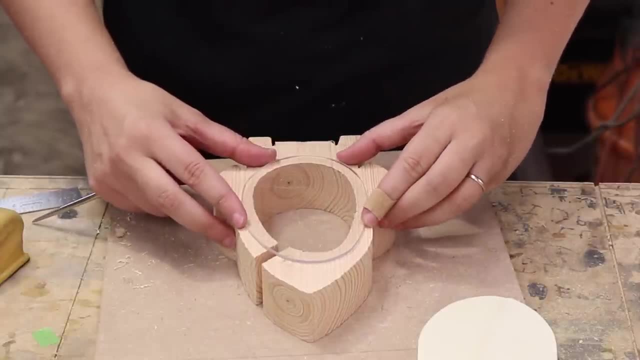 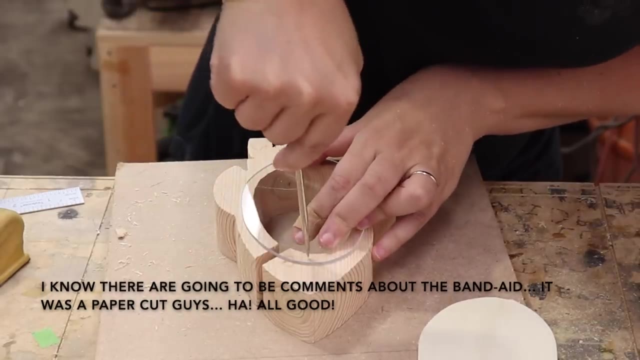 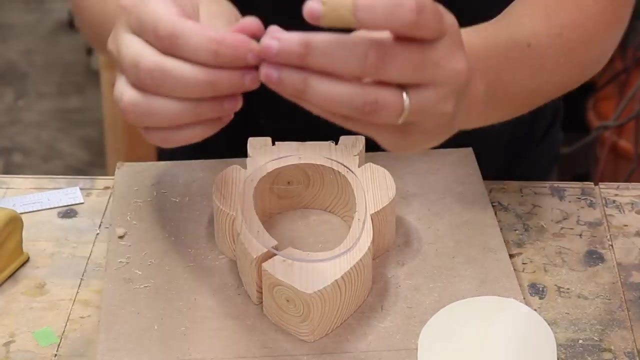 the actual piggy bank part. so now just place it over the hole, make sure there's somewhat of an even gap all the way around, and then use an awl to mark where the screws are going to go- small screws to hold that down. and I just want to make sure that when I'm 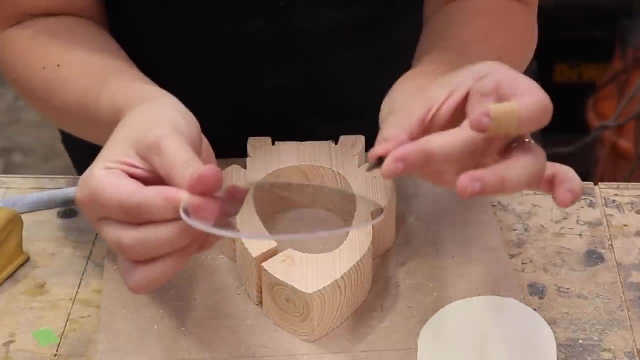 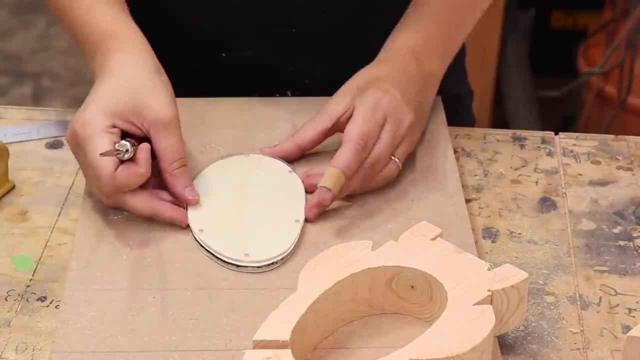 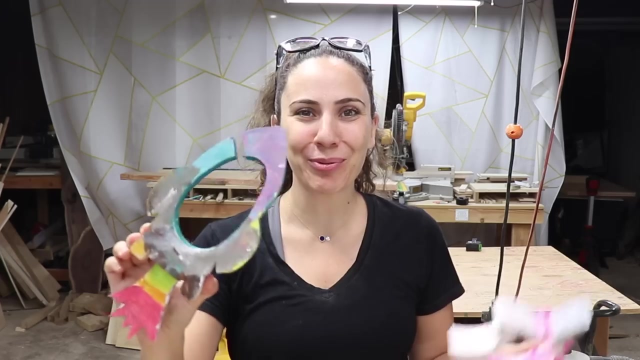 drilling the hole into the acrylic. I'm drilling the hole big enough so that this screw actually fits all the way into it, so that I don't crack the acrylic. now I could just transfer those holes onto the plywood, drill them out all right, cool. so my kids sanded and painted these and it was really fun. my 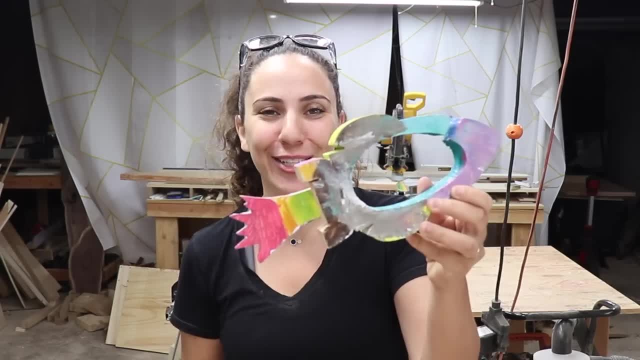 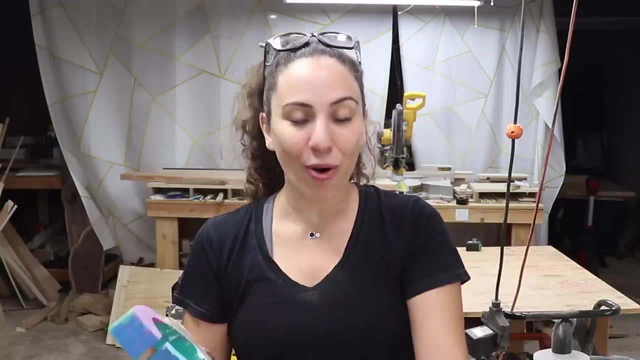 son had an idea to add some fire to the bottom of the rocket ship, which I thought was a great idea. so I cut out a piece of plywood and just glued, and Brad nailed it to the back. so now all the kids need to do is to just screw on. 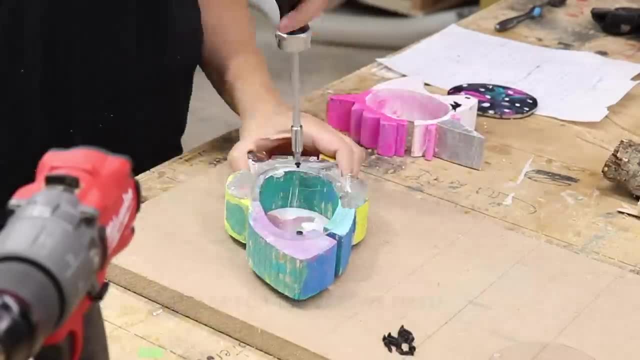 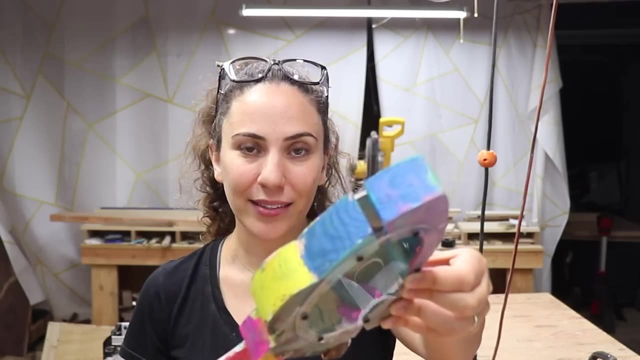 the back plate and the acrylic front, and they love to use screwdrivers, so this is really fun for them also, and it's done so. the way that it works is because you cut a slot in the top. over there you could just drop some coins right in. 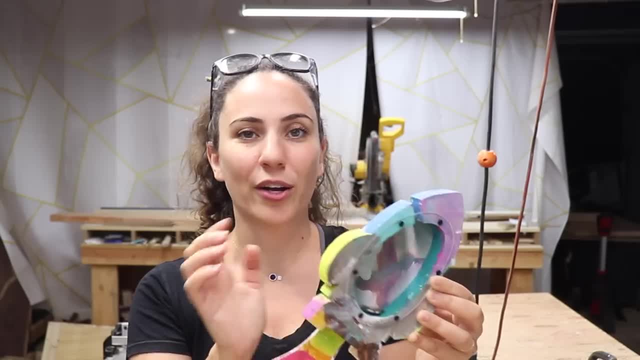 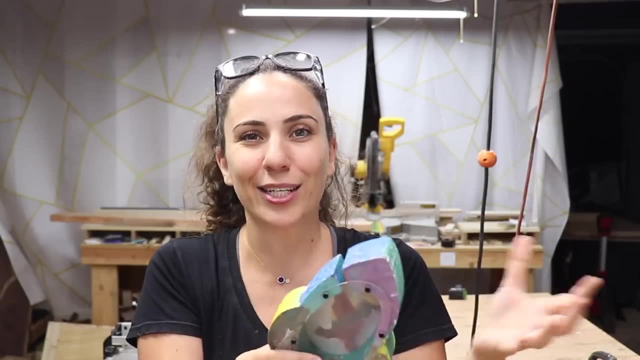 there and when it gets filled up you could either just unscrew the front or the back and take everything out. if you want, you can get a cork plug and to just drill a hole and use that for the back plate and the acrylic front and the front. it's easy enough to just unscrew and screw these back on. this next one is 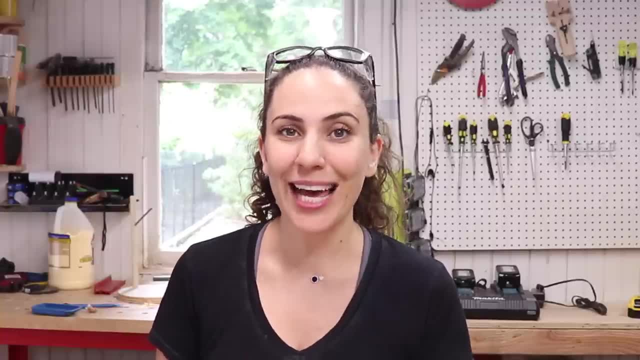 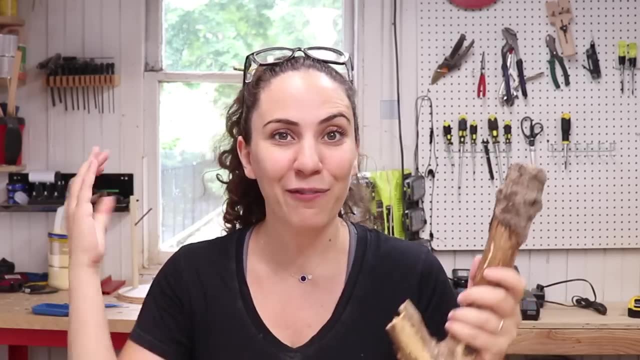 backgammon or checkers in a bag, and what's really cool about this one is that your kids can actually go and hunt for the game pieces in your backyard, so they could go and collect twigs and branches, and that would be a fun activity in itself. I wouldn't suggest anything smaller than an inch in. 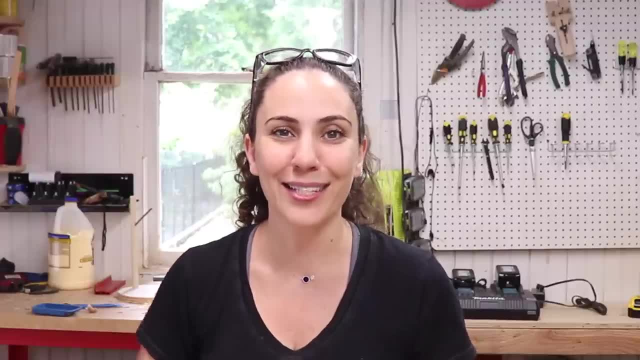 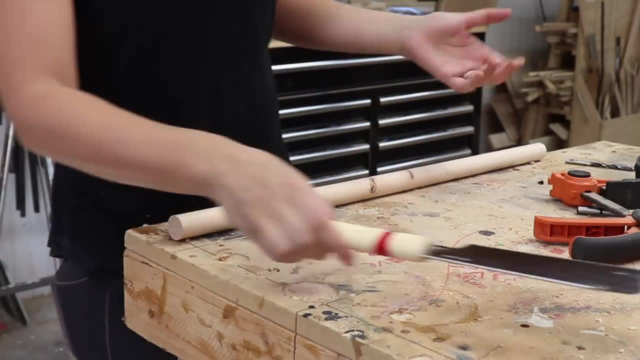 diameter. so just to move forward with this, instead of going to collect some branches, I'll just use a one-inch dowel to show you guys how to make it. once I'm done, I'm going to take a hand saw, and really I'm not going to measure any. 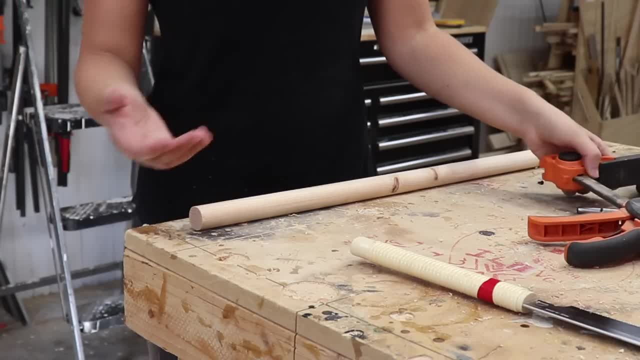 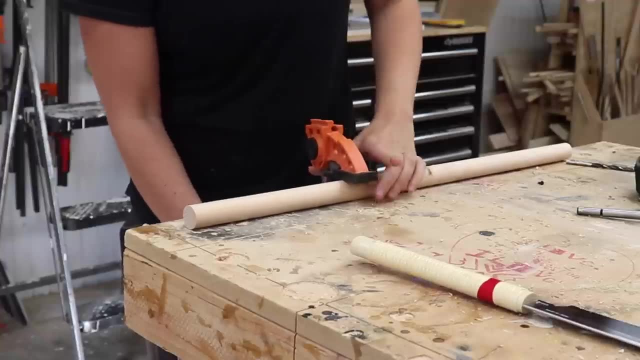 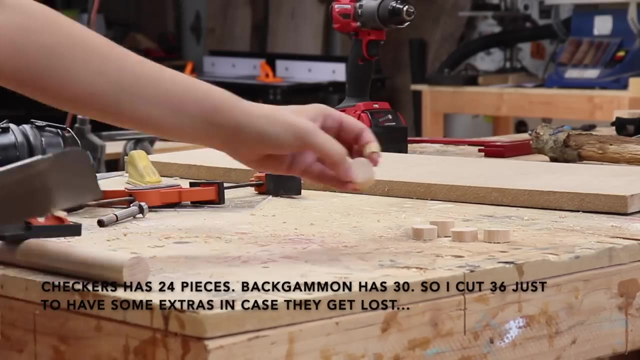 of this at all. I mean, I'm gonna aim for like 3 quarter inch thick pieces, but remember, kids are going to be doing this. it's not going to be perfect and it's going to be awesome because they made it after we send it all the pieces. 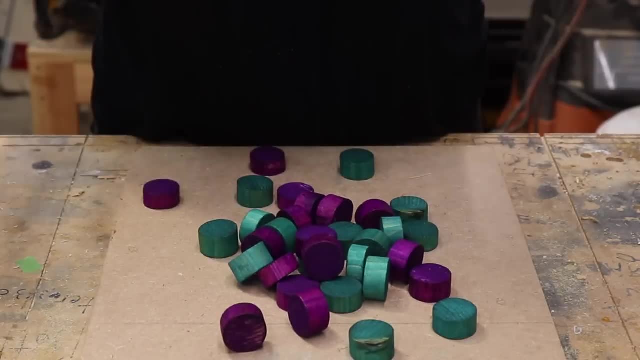 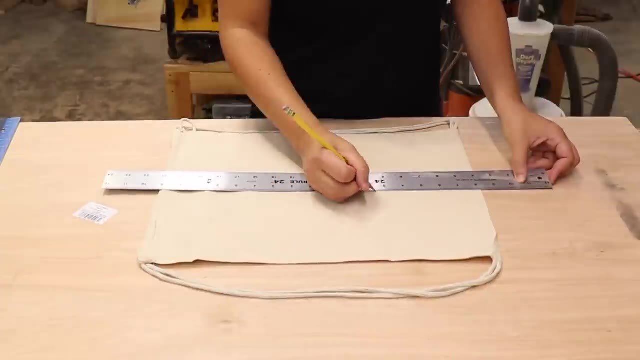 my kids picked colors and they painted them, and for the game board I'll use this canvas bag. so one side I will draw squares for checkers and on the other side I'm going to draw out a backgammon board. so I'm not using a template at all. 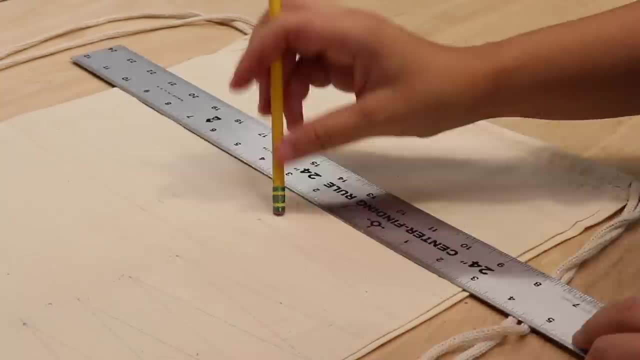 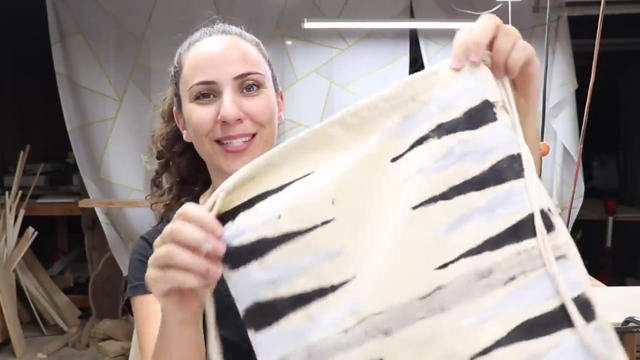 here. I just looked online to see kind of like the proportions and how many things I needed, and then I just marked everything out and then the kids painted it. so one side is checkers and one side is backgammon. so, as you can see, this is. 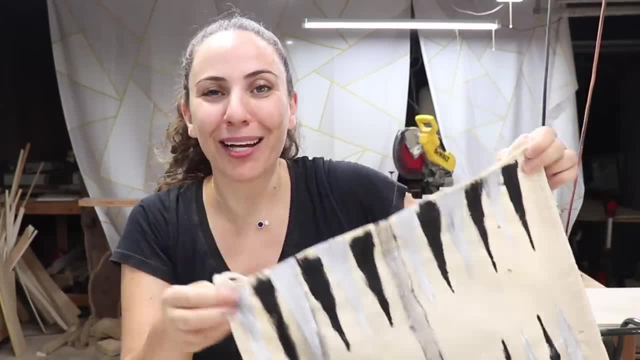 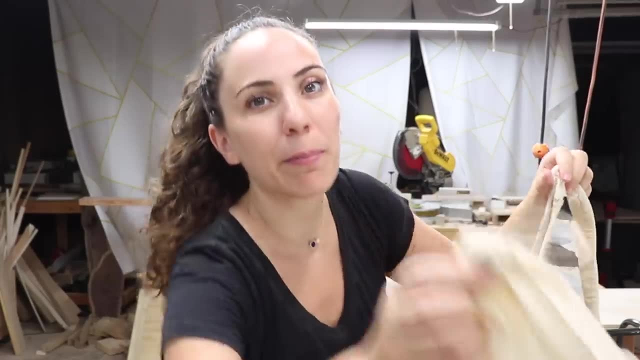 not perfect at all. Mistakes were made, some colors were put in the wrong spots, but it's still just something that they made and it's awesome for them. So, since this is quite a big bag, I wouldn't put the game pieces directly into the bag. I. 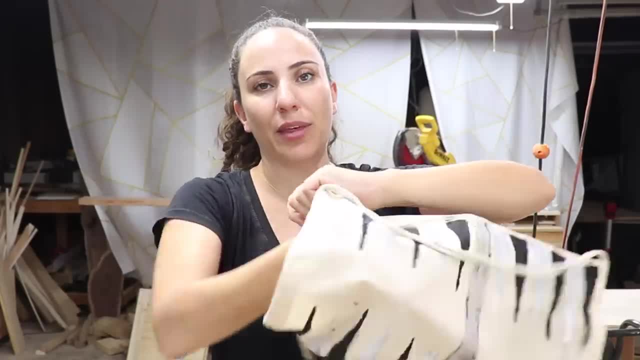 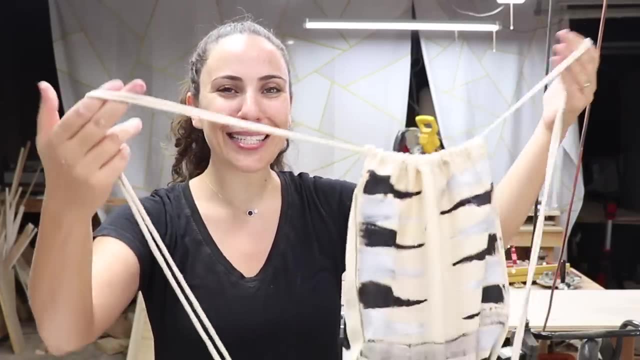 would put them in a little sack first, and then I would put that in the bag so you could just fill this up with some snacks and take this to a park or something, play some games, have some snacks. I think these are really cute. 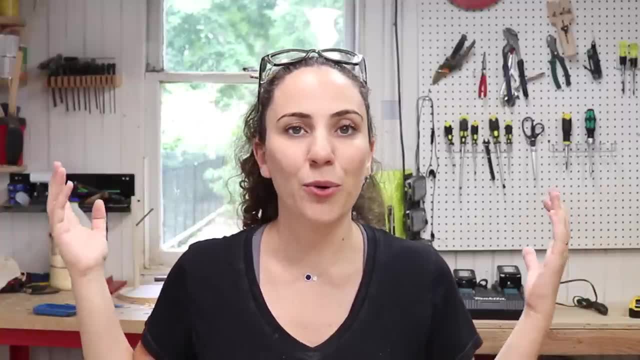 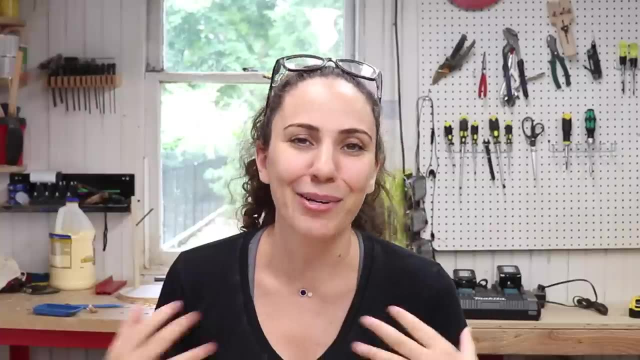 The next one is an analog speaker for your phone. This is geared more towards older kids who either have a phone or who are just into music. So I've seen a ton of pictures of these online, but I've never actually made one of these myself. 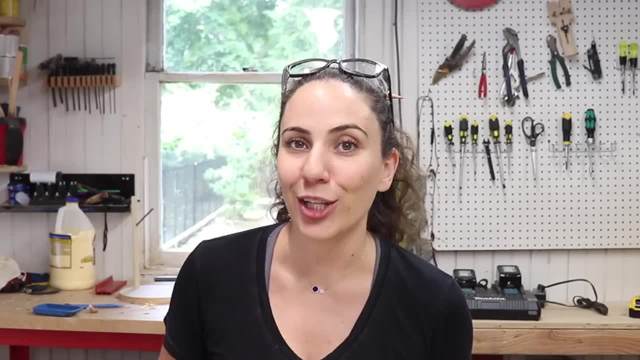 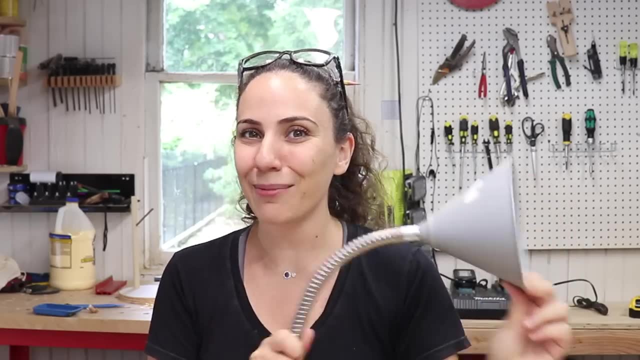 I've been meaning to for a while now, so I'm gonna try to make it look nice with some hardwoods, and I have this funnel that I'm going to use as like the speaker to kind of make it look like a gramophone, and maybe I'll try to make 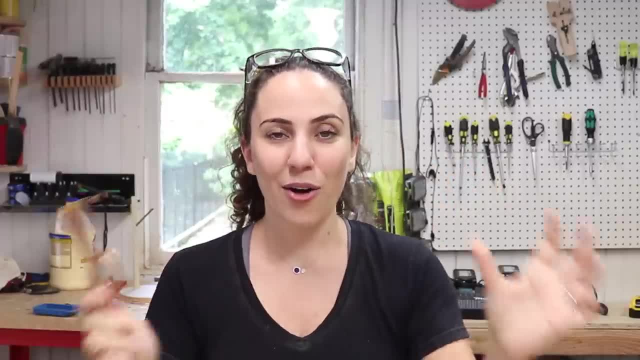 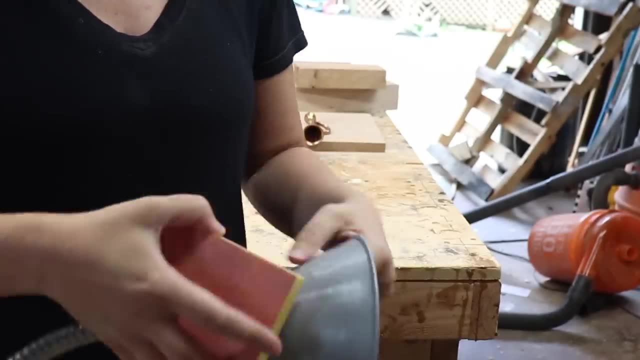 one also with the bugle as a speaker. So I'm gonna try to figure this out on camera and I think this will be a really fun project to figure out with some older kids. Before doing anything to the wood, I just want to prepare the funnel for paint, so I'll sand it, just to scuff it up. so the paint. 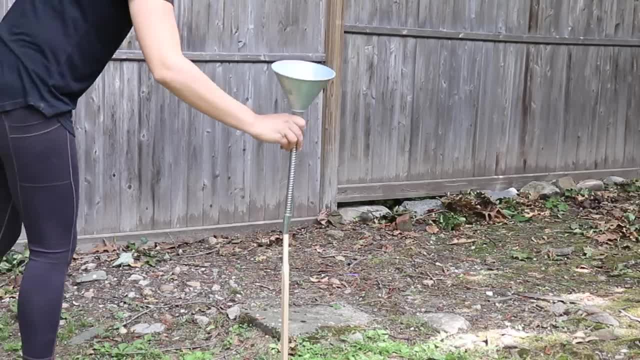 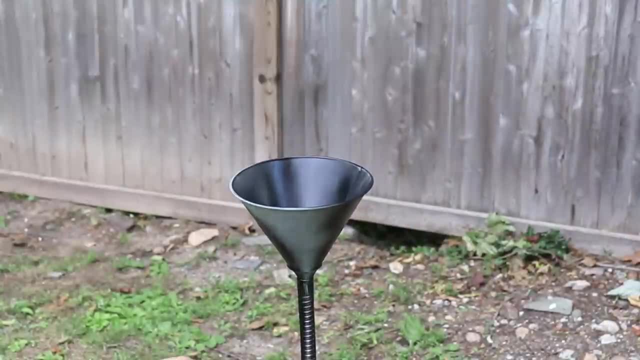 will stick to it. I clamped a dowel into the wood hand screw clamps and then just put the funnel on top of that dowel. I used some black spray paint because I thought it would be really cool as a contrast to the maple that I'm going to. 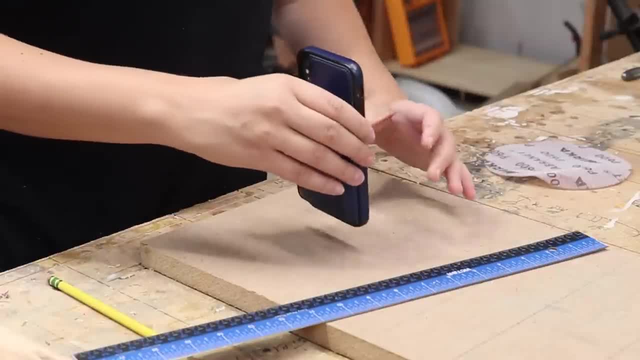 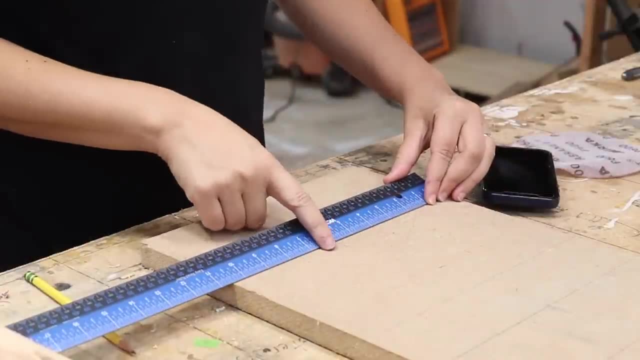 use. The first thing I'll do is measure my phone because I want to make sure it's going to fit with the case on. So I'll just roughly mark this out About seven-eighths. so I'm gonna go with an inch. So this piece is two and a half. 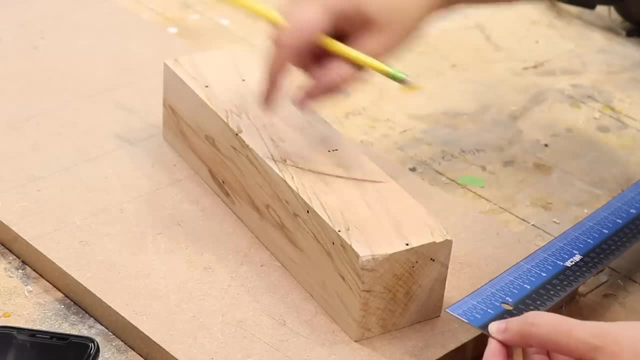 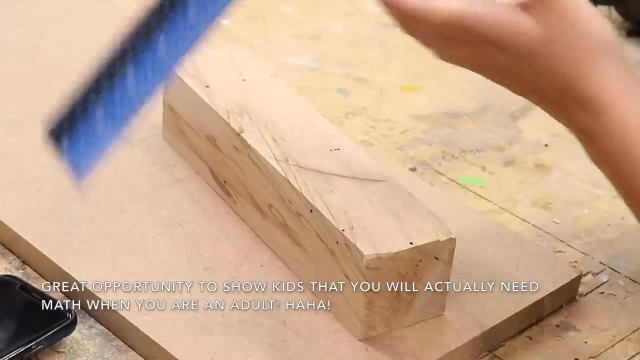 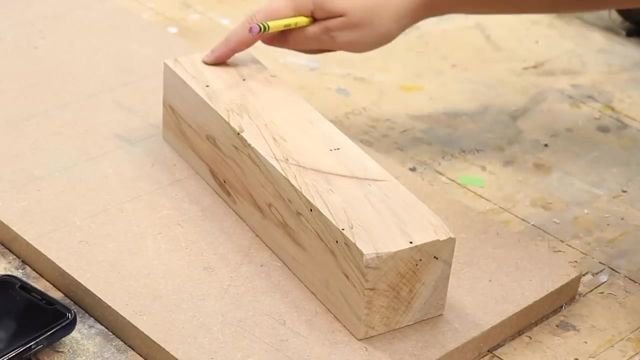 inches wide and I know that I need a one inch channel in the middle to fit my phone. So if I mark three-quarter inches from one edge and three-quarter inches from the other edge, that leaves me with a one inch piece in the middle. So I'll 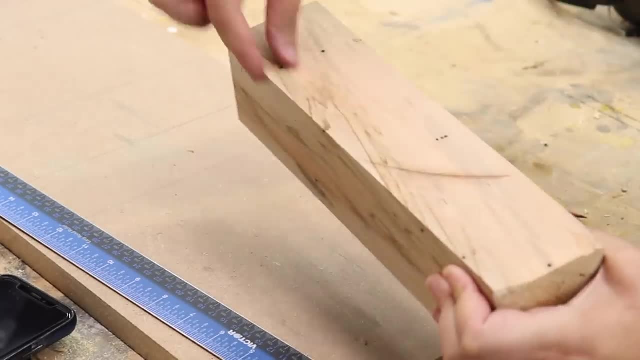 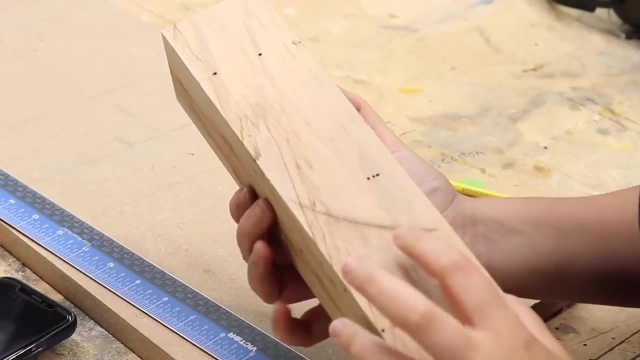 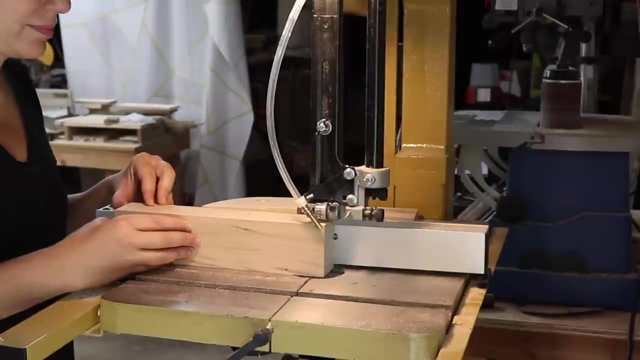 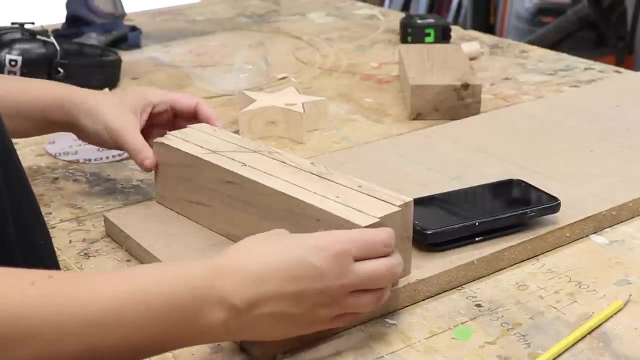 cut this. at the table saw I'll cut two three-quarter inch strips off. Oh, should I use the bandsaw Because it'll be a smaller kerf? Oh yeah, I'm gonna do that. So for the rest of it, I'm just going to eyeball everything. I'm going to 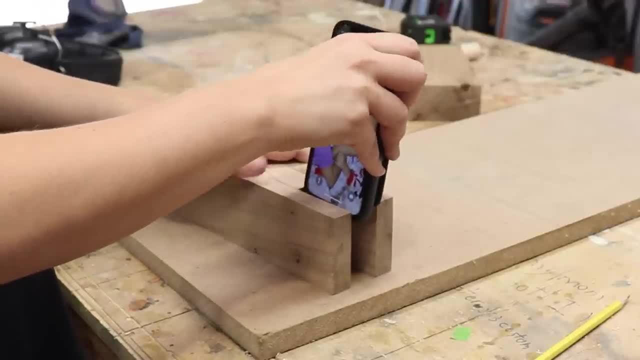 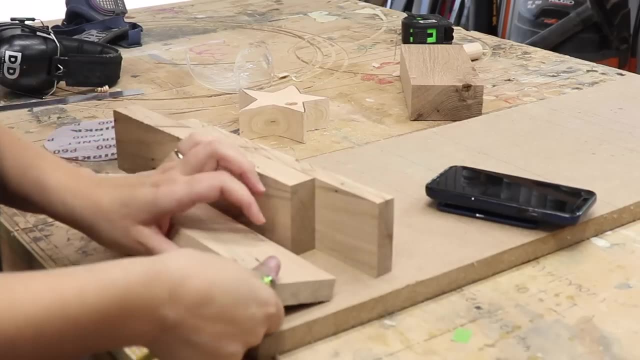 place the phone in here and decide how deep I want the holes to go. I feel like that seems fine, so I'll just mark that on the front of the piece. measure that. so that's also about an inch. where do I want everything to go? so 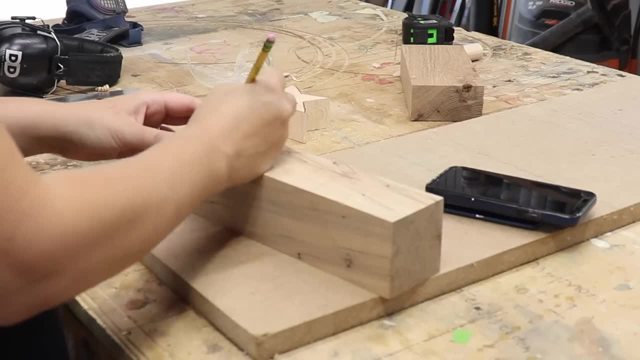 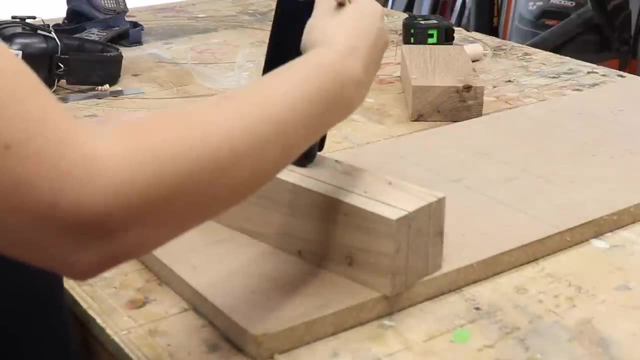 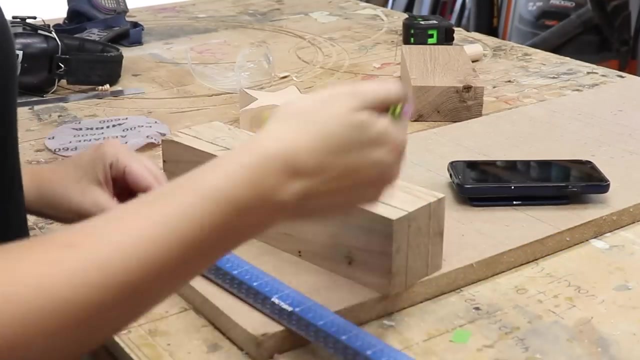 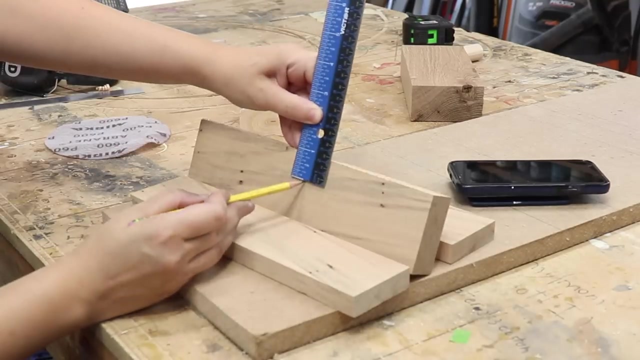 I want the funnel to be like somewhere here. it's gonna be like a circle. that size and phone, just like that, make sense. so mark either side of this. this just so happens to be 3 inches, so 3 inches wide and then an inch down, this little notch. 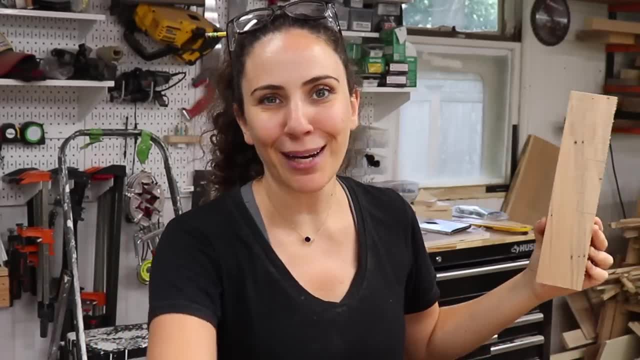 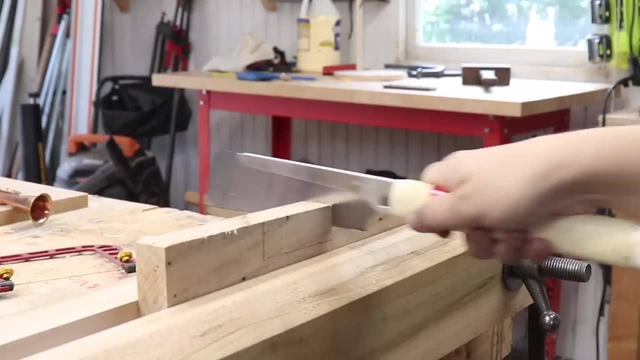 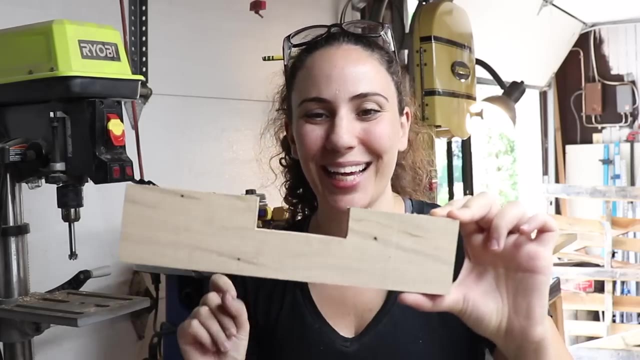 can easily be cut out with a bandsaw. but just for fun I'm gonna do it with some hand saws to show you other ways to do it. sorry, I think my battery died while I was doing that cut, but you get the idea. next I'm going to 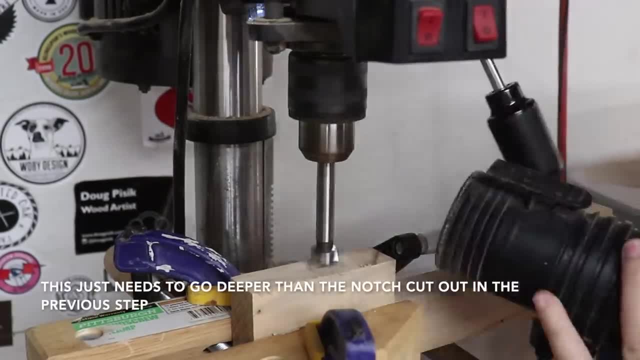 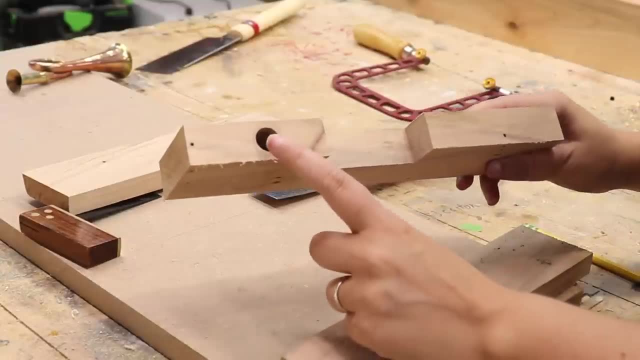 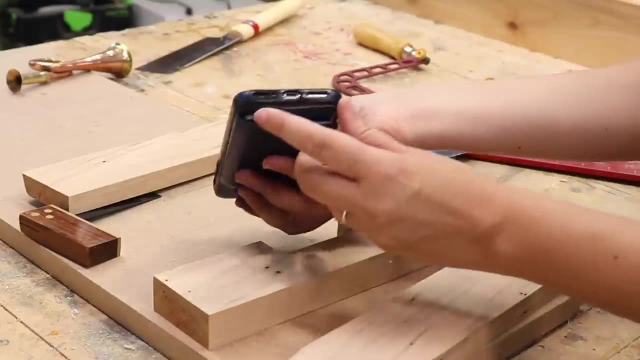 drill the hole for where the funnel is going to go. so now we need to find a way to connect this hole to this area over here. so I want to make sure that it's actually being connected by where these speakers are on my phone, so I'll line up. 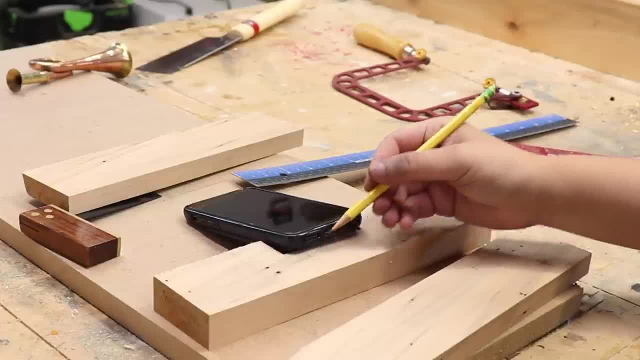 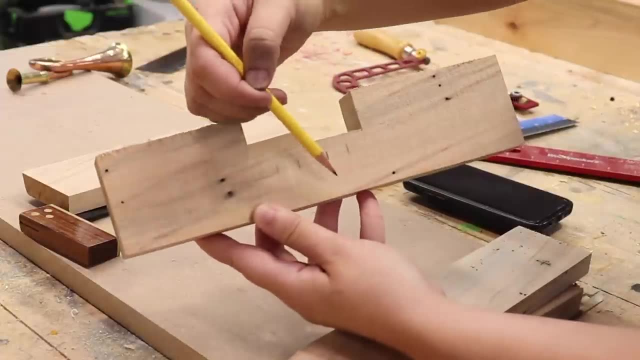 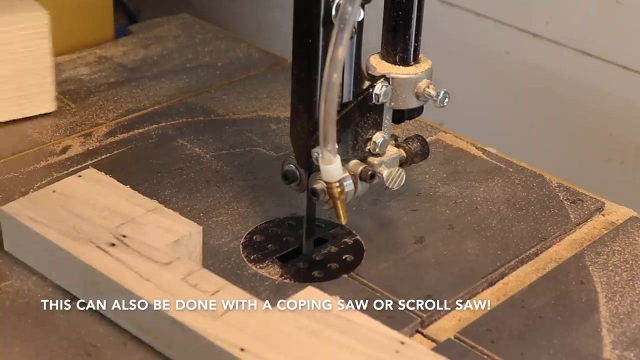 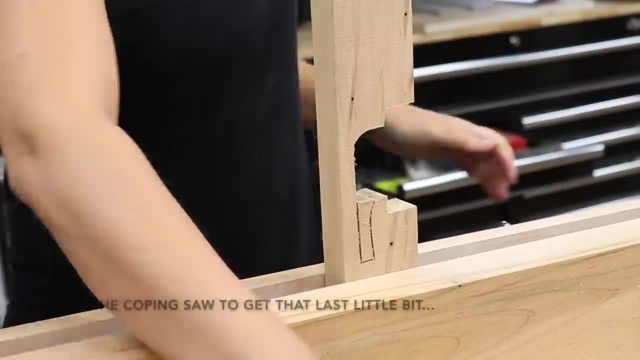 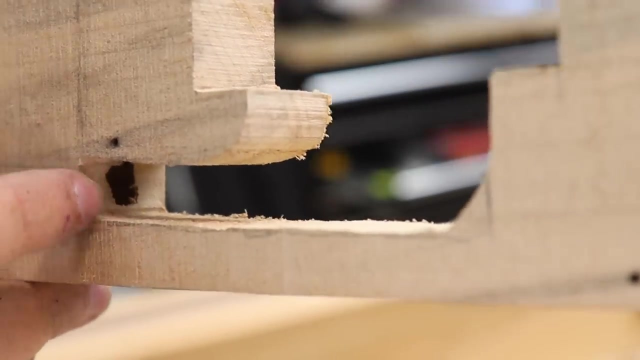 my phone here and I'll mark out where my speakers are. now I'm going to cut a channel that's going to connect these lines that I just drew out to the hole that I just drilled out. now this here is connected to the hole that I drilled up. 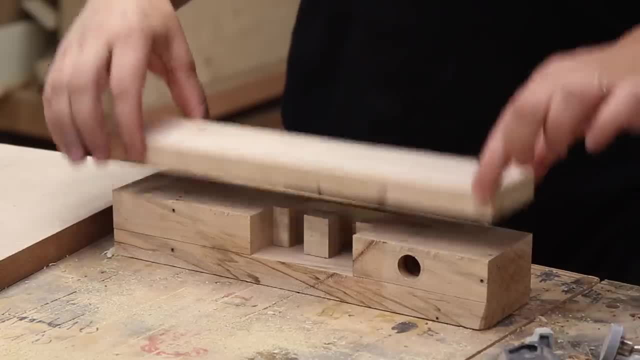 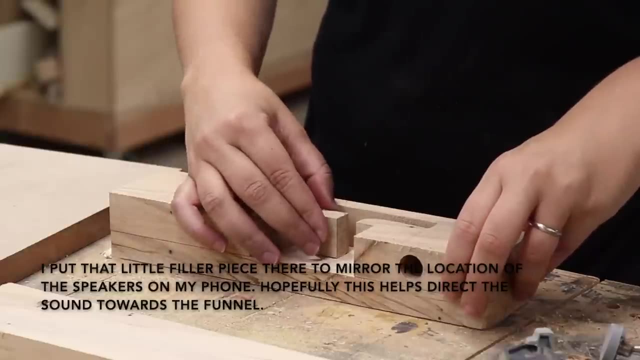 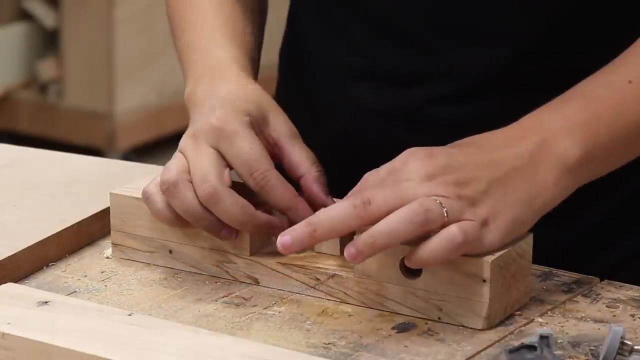 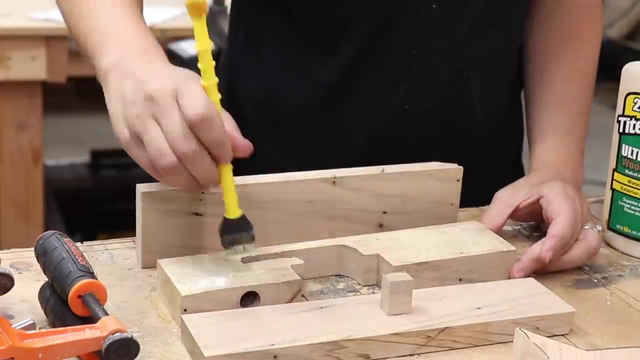 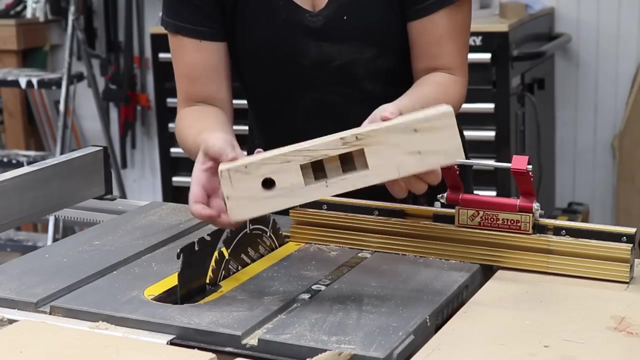 on top before gluing these pieces all back together. I just want to make sure that that little piece is in the right position, so I'll just put it on temporarily with some CA glue on what to one side? okay, now that that's in the right position, I'm going to glue the rest of this up. it's out of clamps and 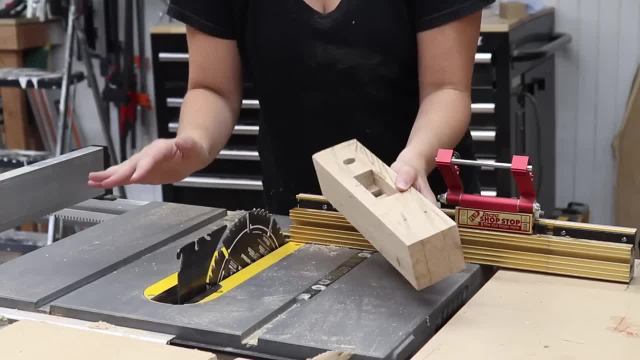 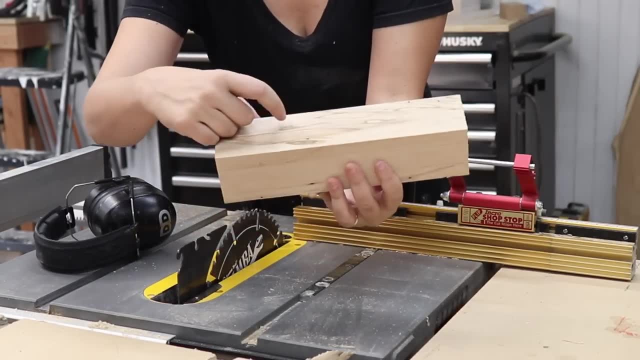 good, now I'm just going to clean up the edges. this is something that I would not let my kids do. this is something that I would do for them. and now I'm thinking on the other end. I want to add an angle. I think that would look really cool. I'll. 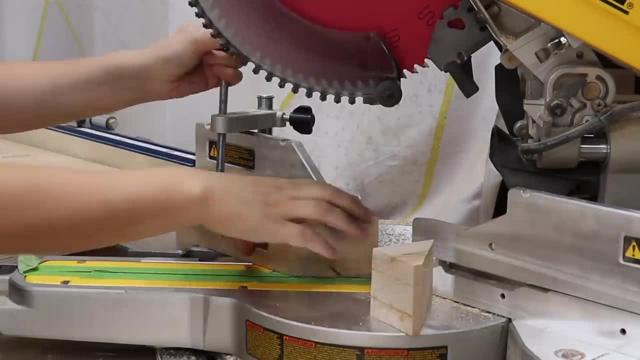 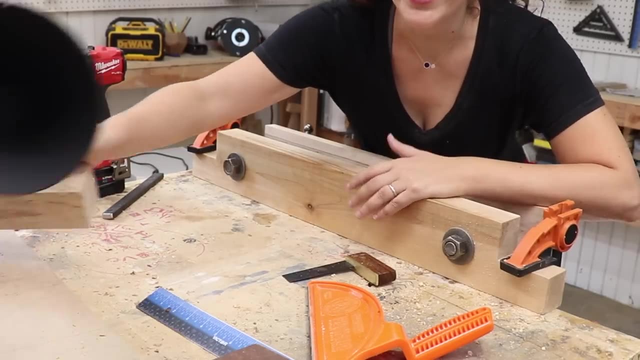 cut the 45 in a miter saw. this is clamped really well. again, I would not let my kids do this. I'll use some five-minute epoxy to glue the funnel into place. so a little bit of a design flaw on this guy. this piece is not heavy. 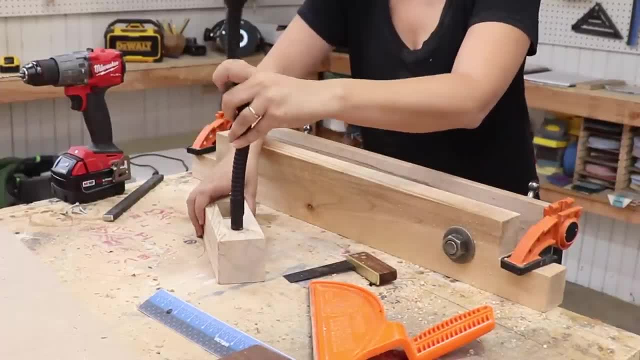 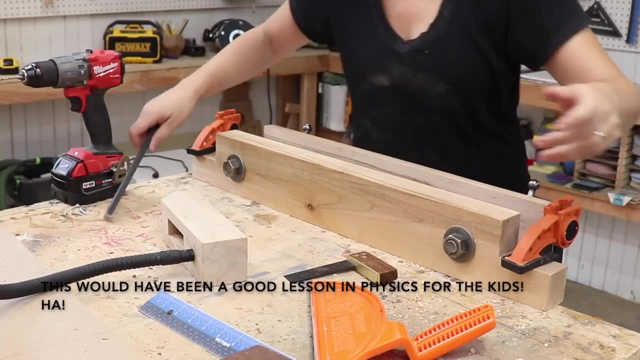 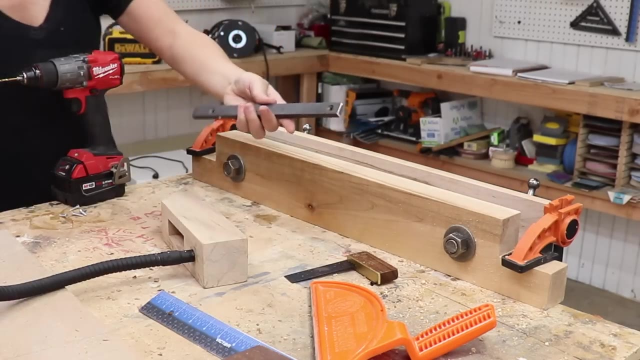 enough to keep this stem in place. so if it's straight up it's fine, but if this is bent forward it tips. so I have these pieces of metal from a crosscut sled track or something like that and I'm just going to screw them to the underside of the base and hopefully that. 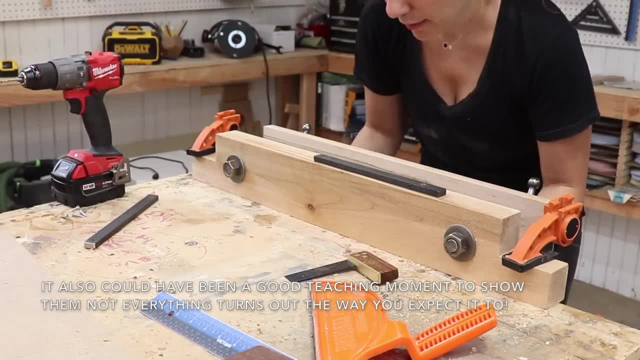 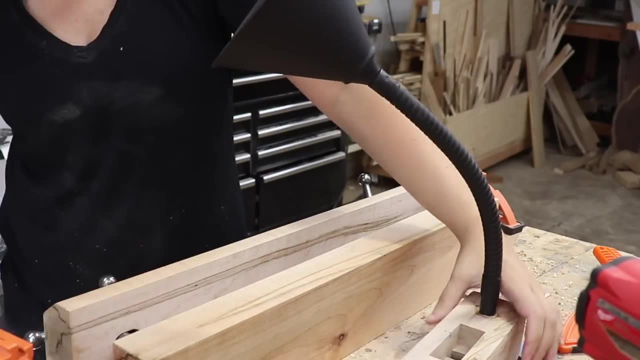 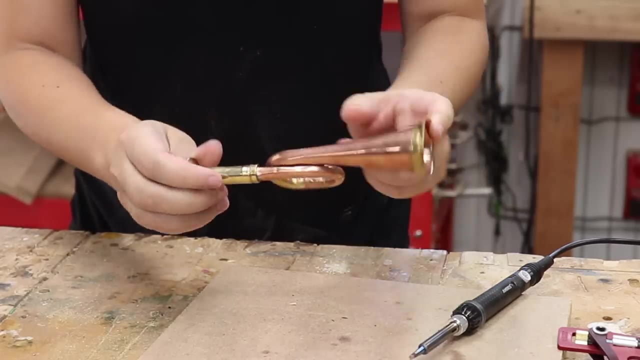 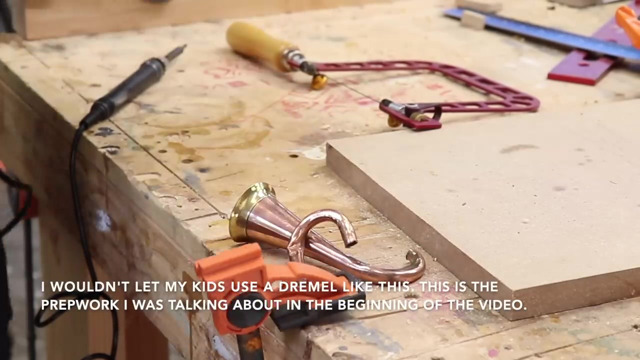 will keep it down so it doesn't tip. oh yeah, okay, it's cool that the black is showing underneath also. oh, I like that awesome. the next one: I'll try to use this toy bugle as the speaker and I just want this curvy part like right there for this one. I want to see if I can make one. 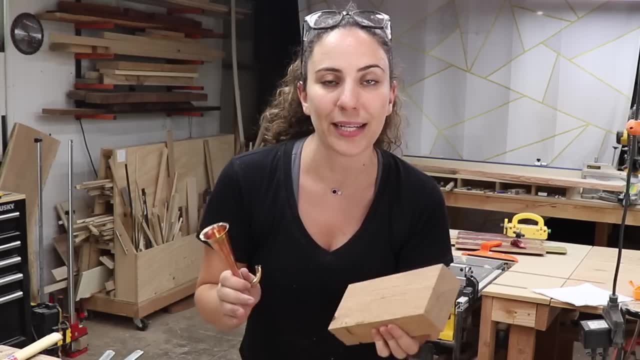 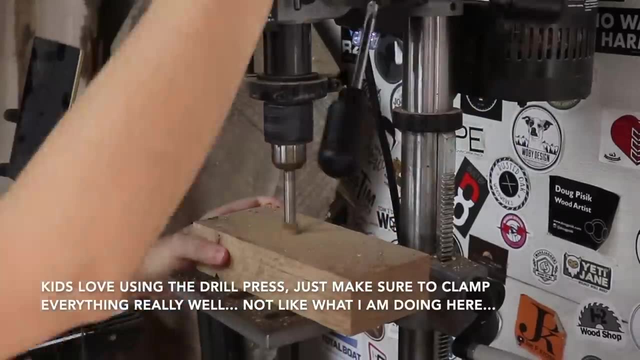 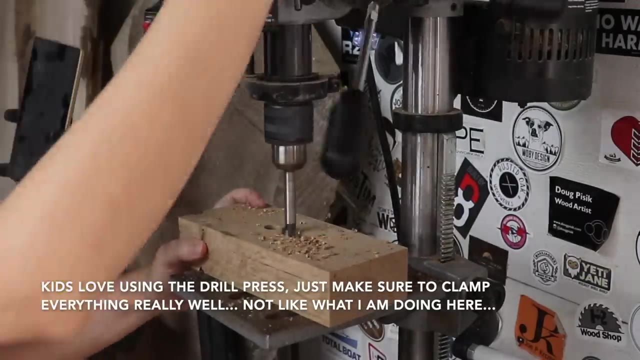 without having to rip the wood and then glue it back together. so I'm just going to try to attempt to drill some holes to create all the sound connections. first, I'll drill out a row of holes that are at thick as my phone, and I'll drill them to a depth that's about like a half inch. 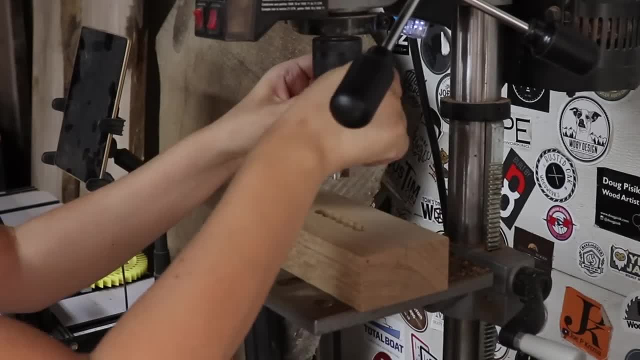 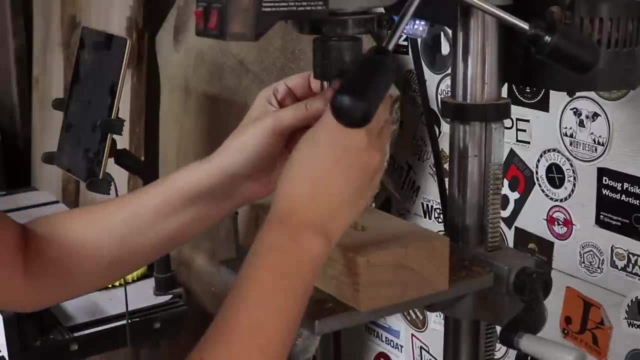 deep. While I'm already at the drill press, I'll switch out the bits to a quarter inch bit and this is going to be for the sound holes, and I'll make this just a little bit less wide than this and I'll make sure that it's in the 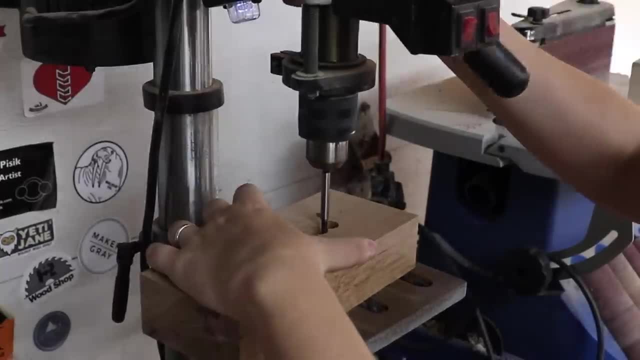 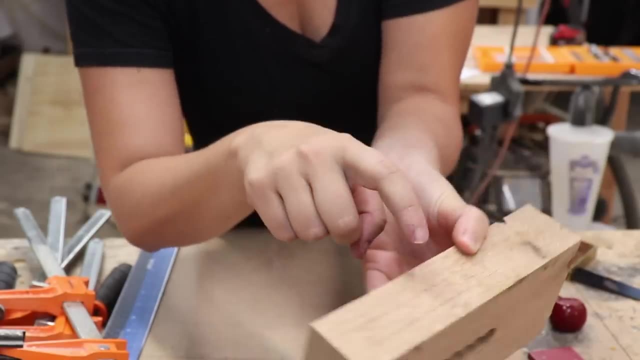 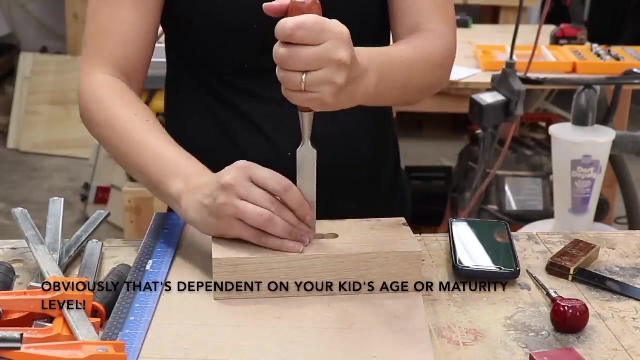 center. It was hard to see what I was doing at the drill press there, but here there's bigger holes and then smaller holes that are less wide but go deeper into the block. Now this is a great opportunity for kids to practice with some chisels. 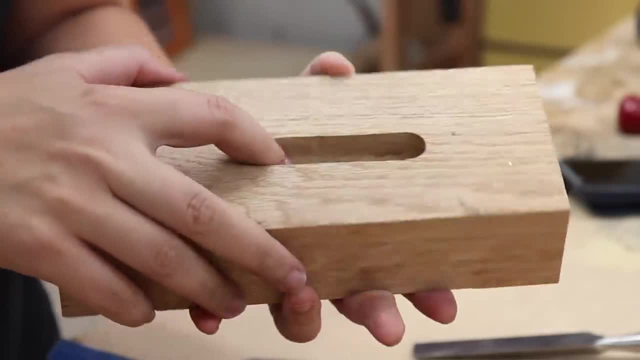 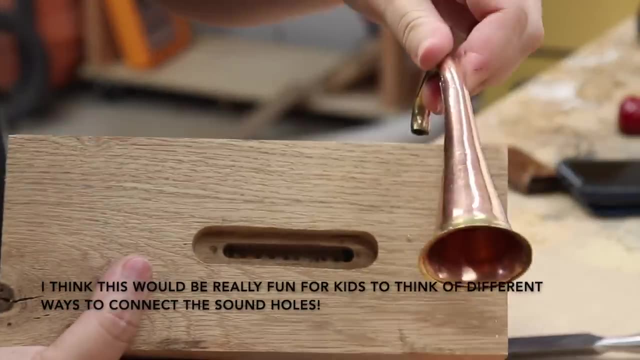 Now I have a stepped mortise in here and I need to figure out a way to connect to that bottom lower skinnier mortise to a hole that I'm going to drill for this. So I think what I'm going to do is 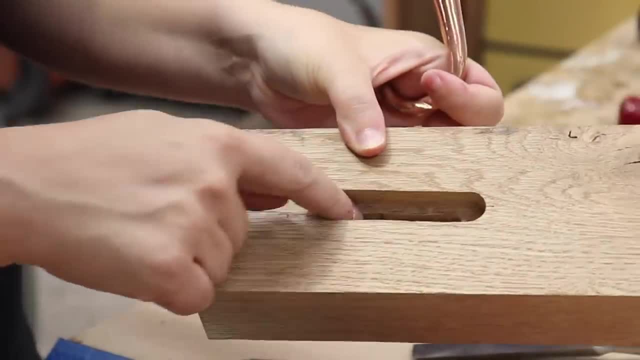 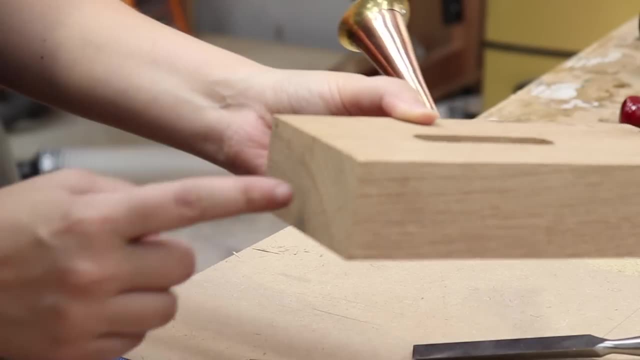 drill the hole for this at the same depth as that lower mortise part and drill it until I get to the end there, and then I'll come in from the end grain and drill the same size hole this way until I connect to the bottom mortise. 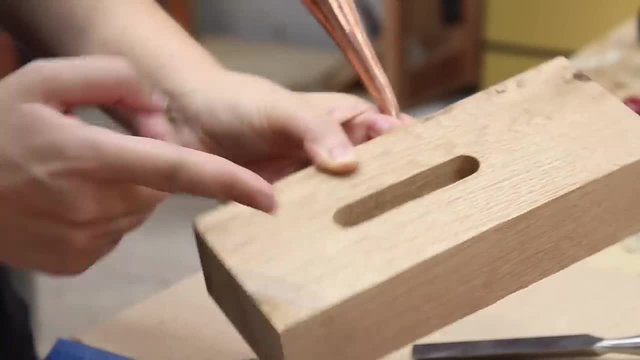 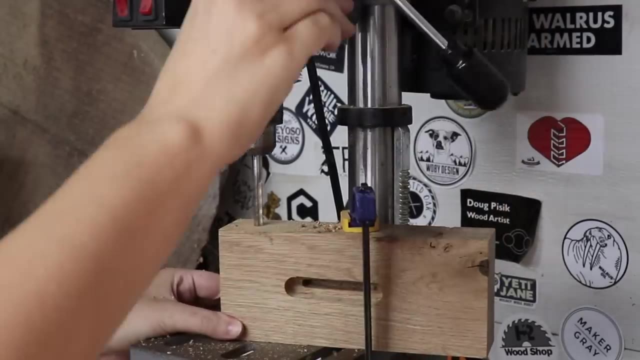 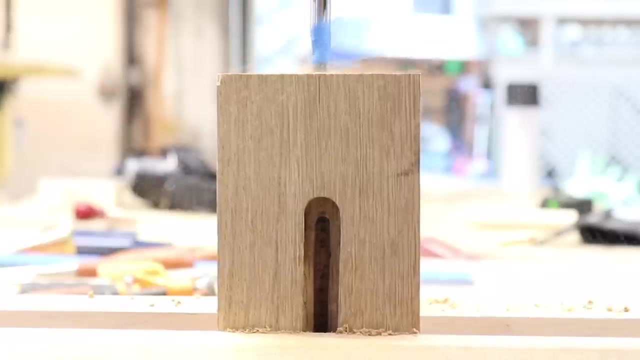 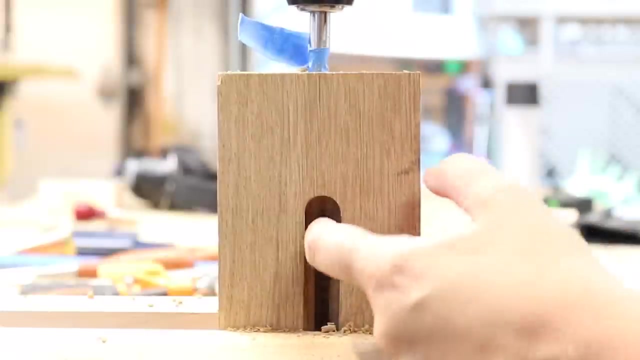 here, and then I'll plug that up with a dowel up until it gets to this line. So I think that's gonna work. Let me try that. Alright, Is it connected? Yep, See the drill bit right in there. So this hole is now connected. 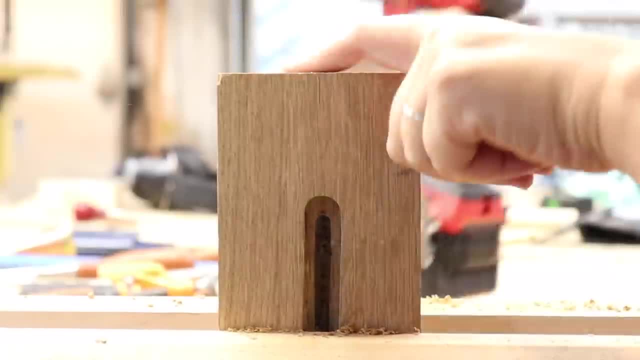 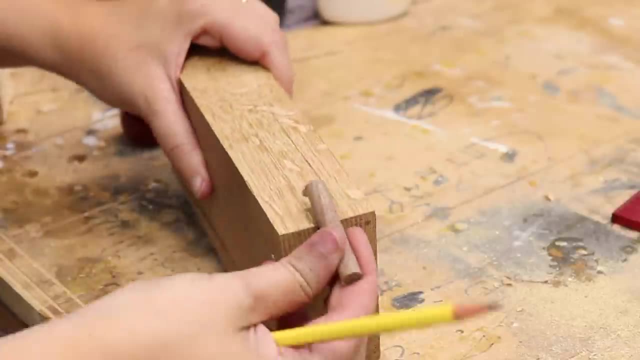 to this hole that's back here and now I'll just plug this up up until this back hole with the dowel. I want to make sure that I'm not going to go deeper than this hole over here, because then that's going to block the sound. 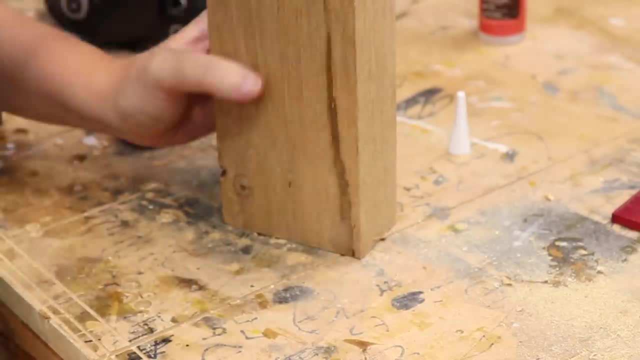 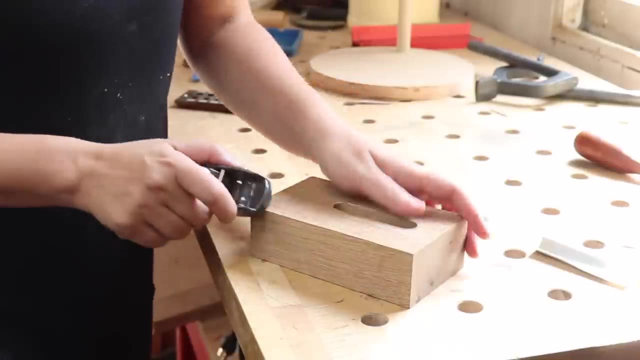 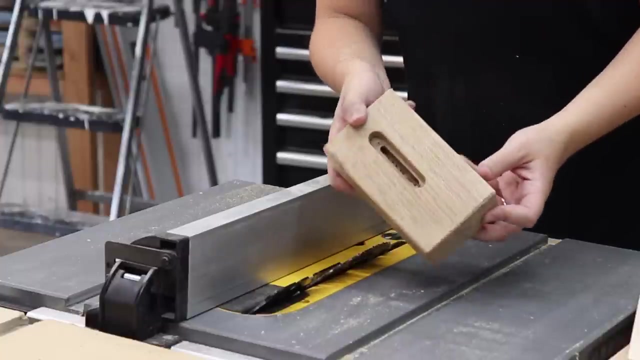 I cut the dowel flush Now. another thing kids love to use is a block plane. They just find it really satisfying to see the shavings come off of these block planes. They're really fun to use. This looks cool as it is, but I think it would be even cooler if there was. 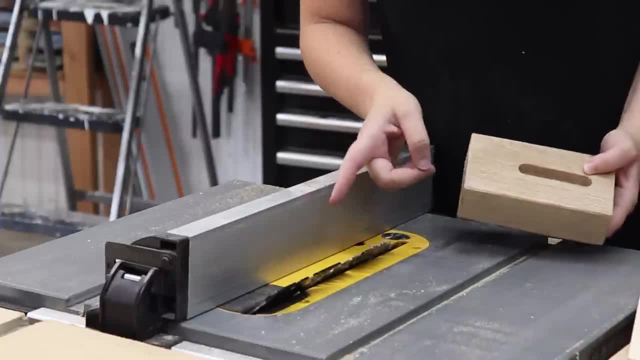 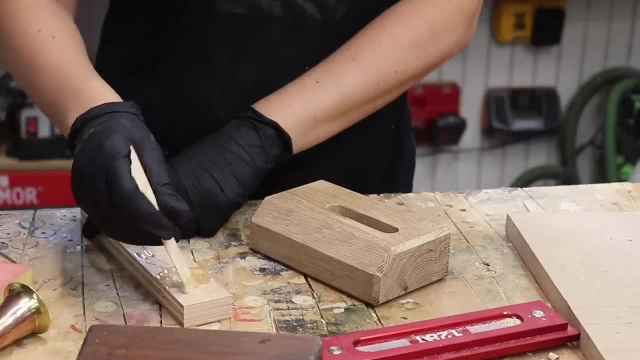 like a deep bevel on the front edge, So I'm going to do that on the table saw. I wouldn't let kids do this. This is something that an adult should do. I'll just use some 5 minute epoxy to set the horn in place. 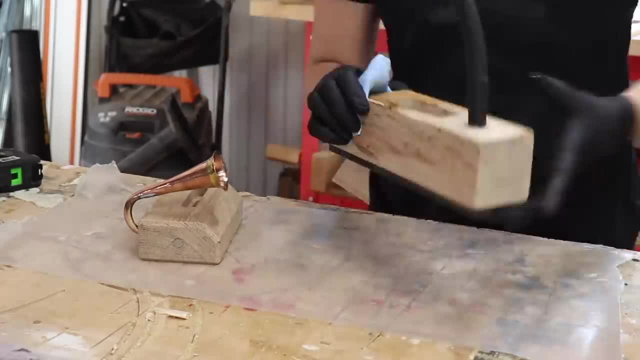 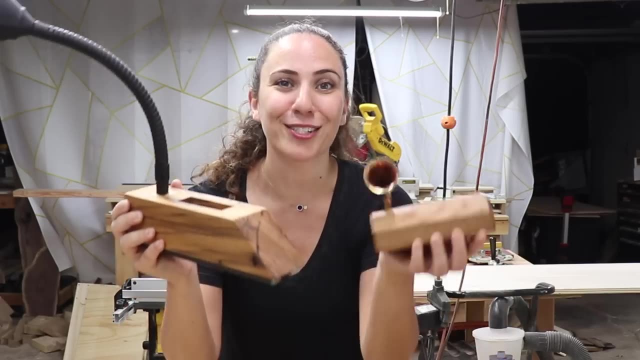 No paint on these guys. Since it's a hardwood, I'm going to finish it with a furniture finish. This happens to be all natural and it's really safe for kids to use. Okay, so these are super cool. So much fun making these and I think it would be so fun. 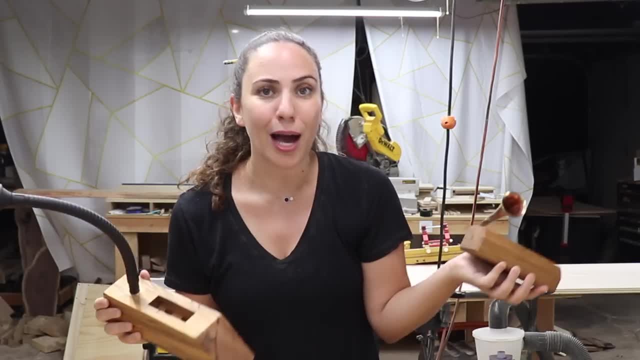 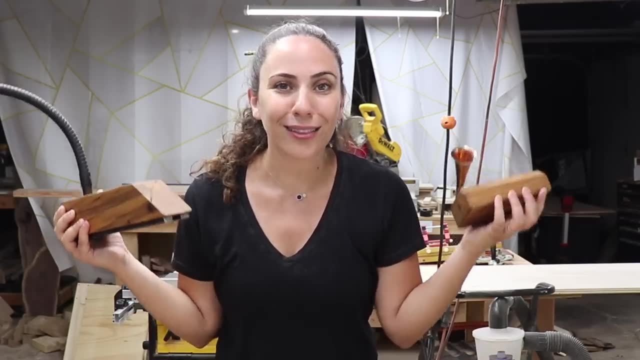 to hear kids ideas on how to connect the sound holes. I'm sure that they would come up with some crazy ideas. You could test them out, see if they work. It'll be like a whole science experiment. Love it. So this one ended up. I had to add the metal on the bottom to keep it standing and that 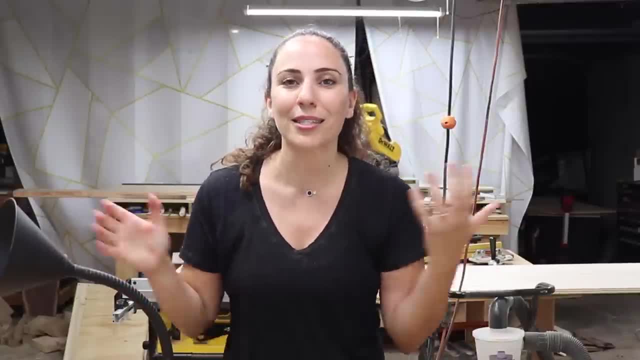 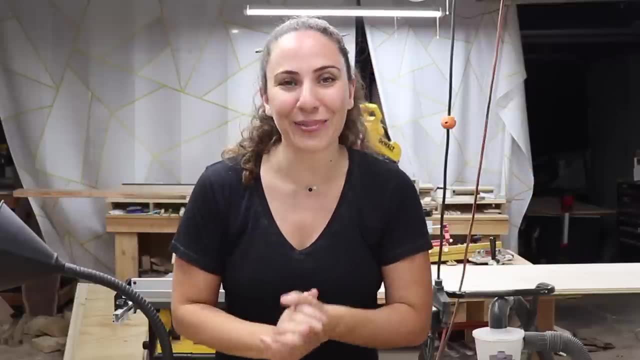 could have been a great learning lesson for them to see like: oh, you should have thought to use a heavier bottom. Yes, I should have. So I want to test these out. I'm going to have to find some royalty free music. Hold on one moment, I'll put it on full volume. 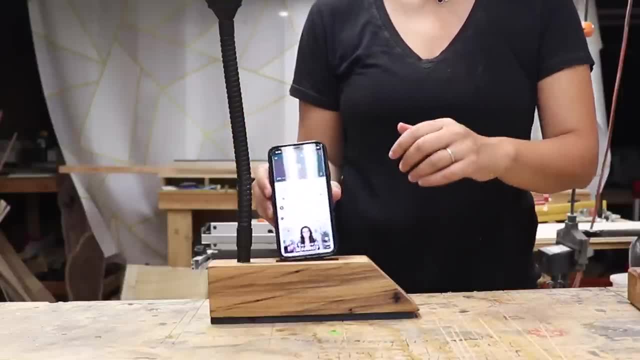 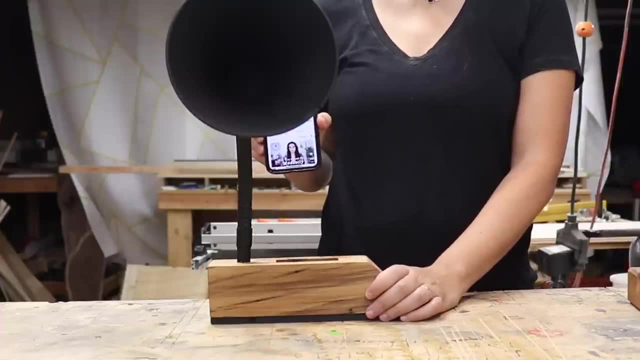 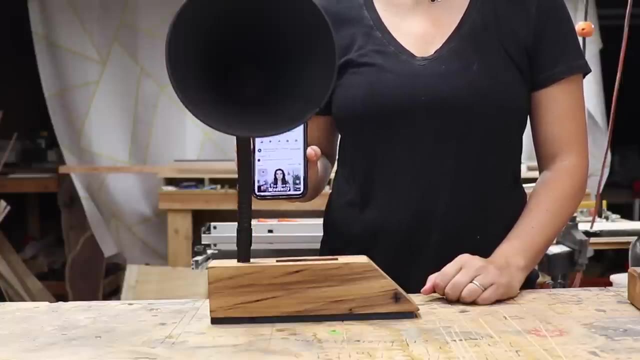 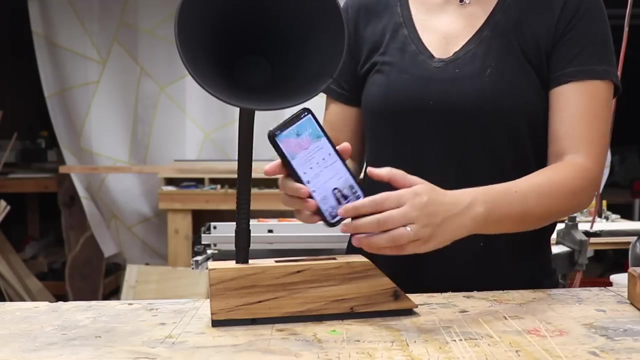 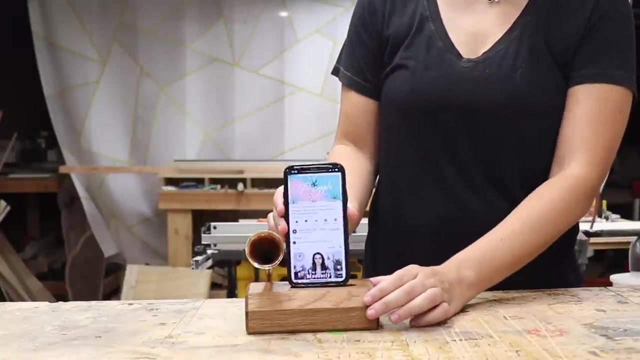 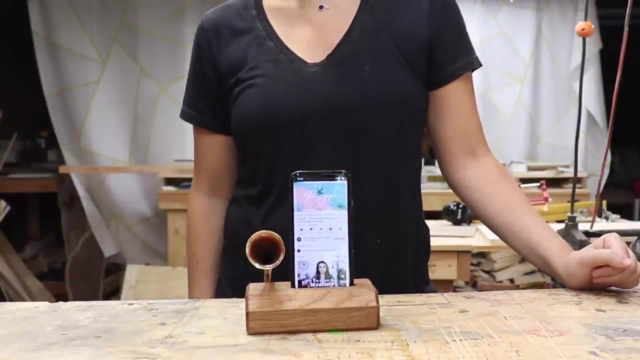 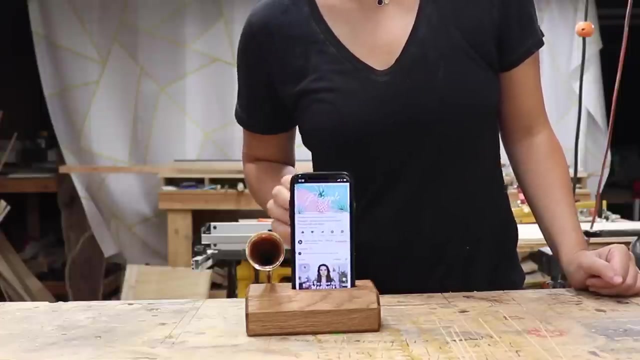 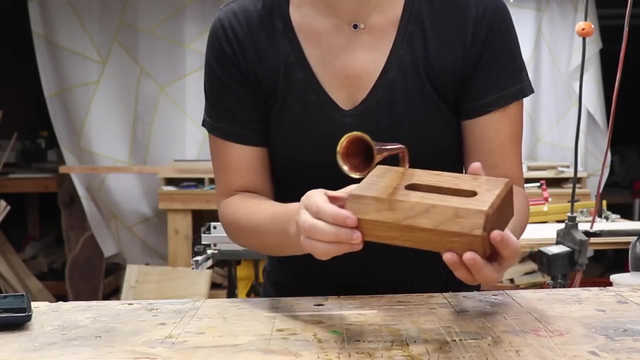 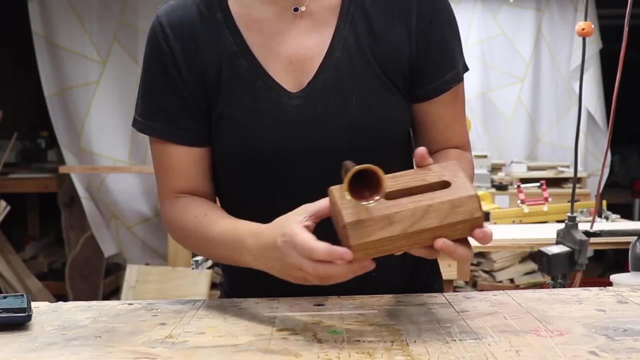 to see if you guys can hear the difference. It's kind of cool that the directions can be changed also. Alright, next one: cool. so this one's definitely not as loud. it's just more projecting in one direction over the other, which is just kind of cool. it's kind of directing the sound. it'd be really cool to go.